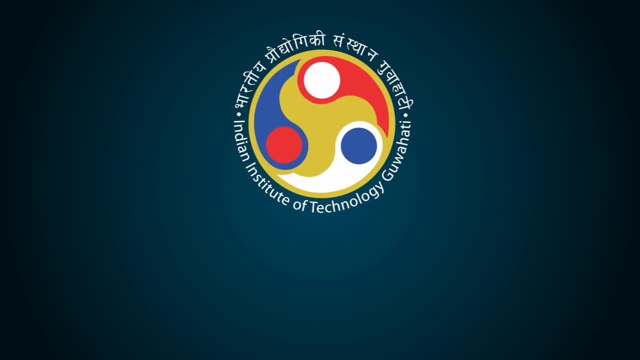 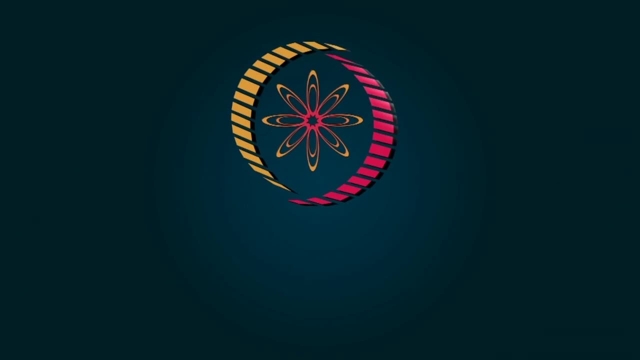 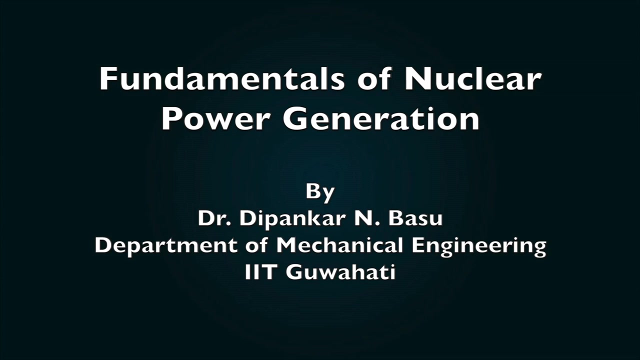 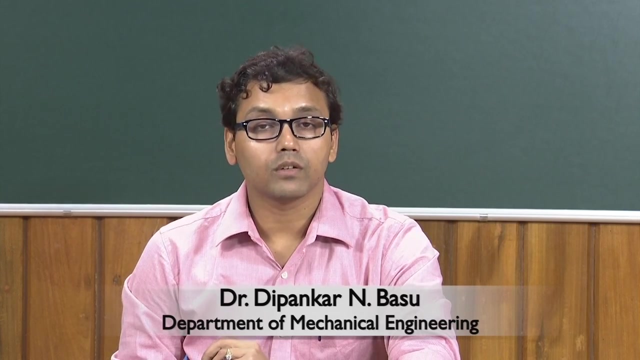 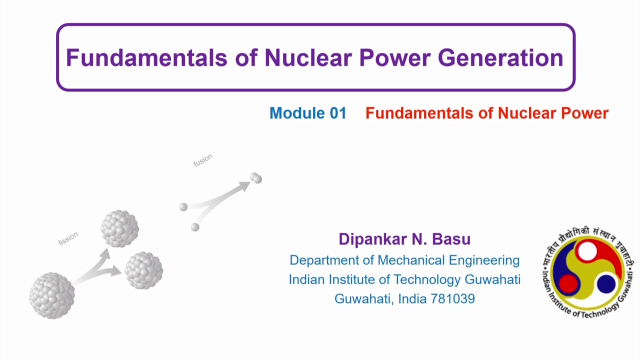 Hello and welcome to this CSS MOOCs course entitled Fundamentals of Nuclear Power Generation, which has been offered under the NPTEL online certification scheme. I am Dipankar Narayan Basu, Assistant Professor in the Department of Mechanical Engineering, IIT Guwahati, and I am going to. 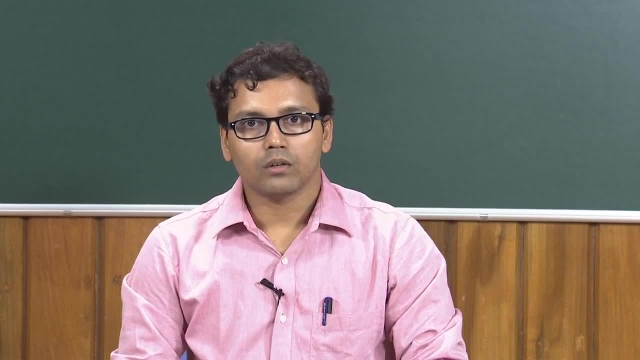 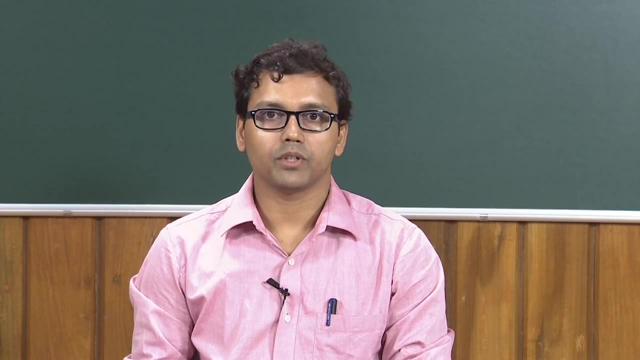 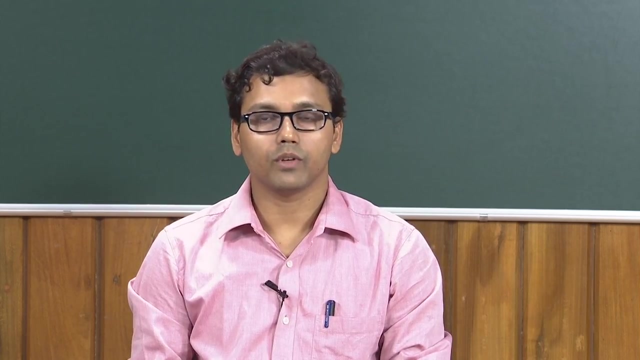 be your instructor for the entire of this course. Now, the, as I have already mentioned in the introduction video, that the topic of nuclear power generation is a bit of advanced level topic and therefore I would expect the entire audience of mine to be either at the advanced level of your undergraduate curriculum or 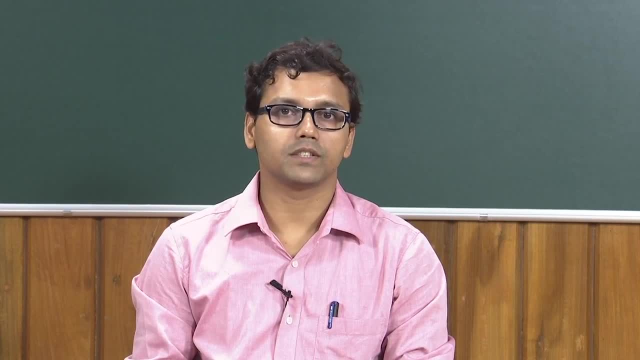 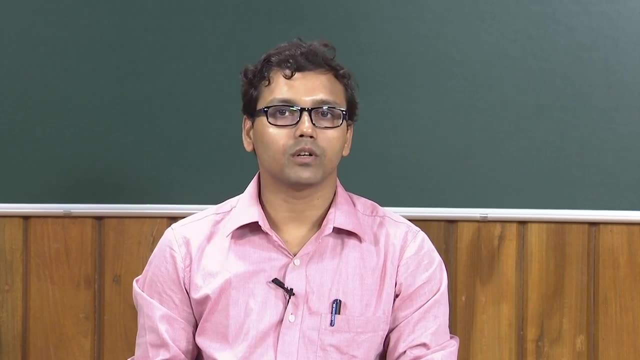 maybe doing a post graduate- that is, you must be at least at the sixth semester of your UG course- or maybe doing a master specializing in mechanical, thermal or nuclear or power engineering, So that you already have the fundamental knowledge about fluid mechanics and heat transfer. 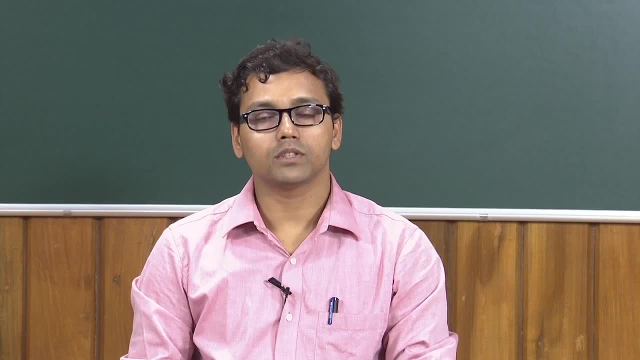 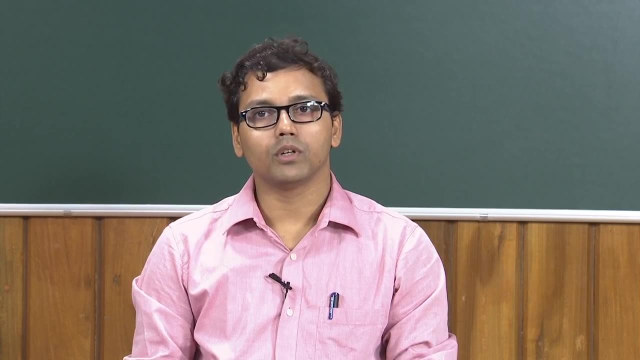 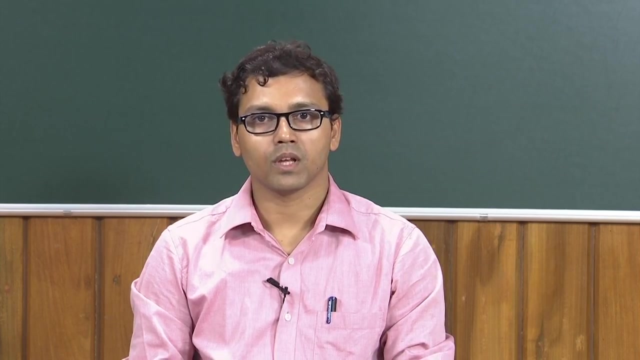 And also you are aware about the laws of thermodynamics and also you are quite aware about the differential calculus or differential equations. rather, because we need to make use of those concepts, some of those concepts, in different sections of this particular course, It is quite a bit odd for me that there is 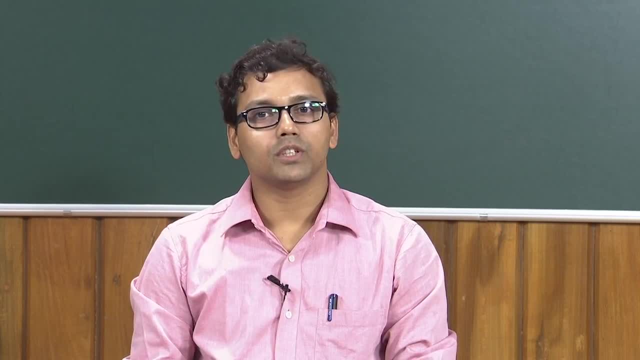 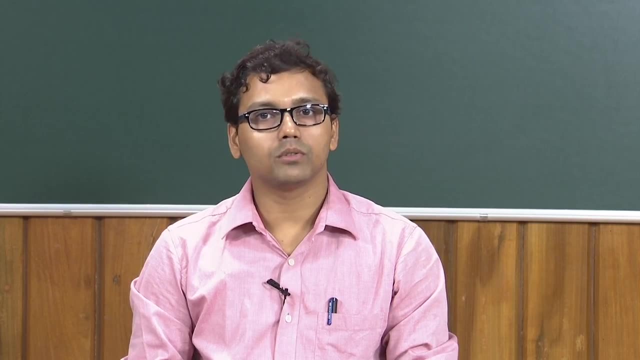 no audience in front of me and I am not even a position to have a direct interaction with you or have eye contact with you, face your questions directly, But still I would like to keep this course as much interesting as possible, Interacting as I can, so that that means I would like to follow more questions as a 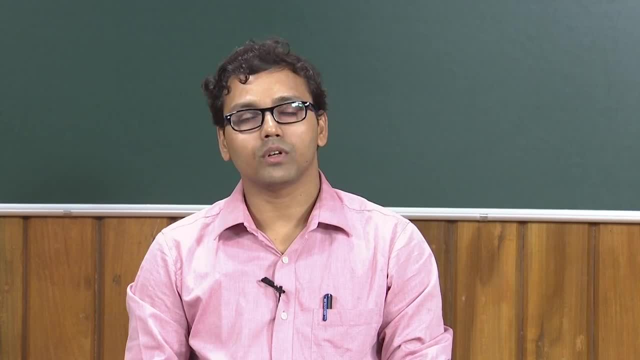 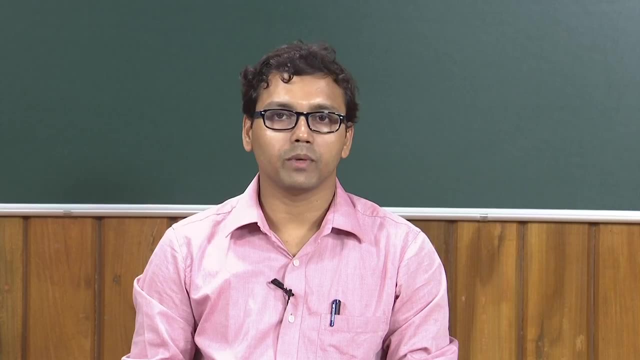 kind of pattern. So, and I am sure all of you are going to respond, that is, whenever you have any query or any doubt or you need any clarification, do not hesitate to drop a mail to me. I would try to respond to that at the earliest And for that purpose while 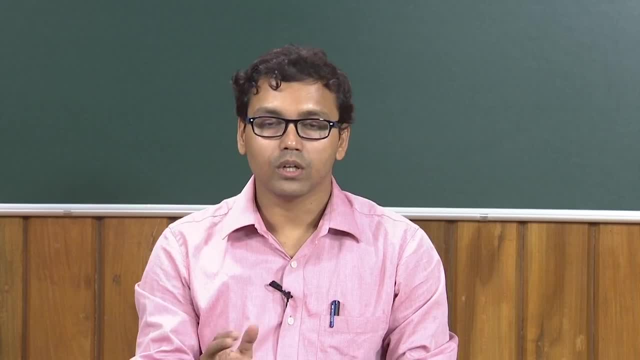 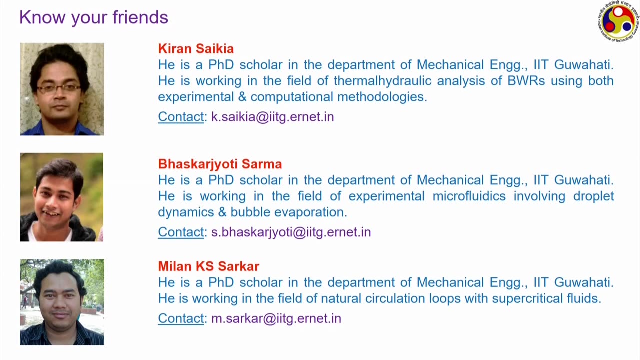 my contact details are already available on the course webpage. you should also know the phone number of my friends. that is my TAs. I have 3 PhD students as my TAs. all of them are quite senior PhD scholar in the. 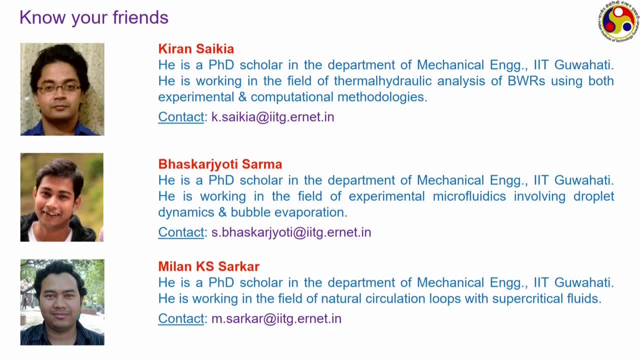 Department of Mechanical Engineering, IIT Guwahati, Mr Kiruksaikeya, who is working in a field of boiling water reactors and therefore his PhD topic is quite relevant to the content of this course. Mr Vaskarjithi Sharma is working on microfluidics and heat transfer. 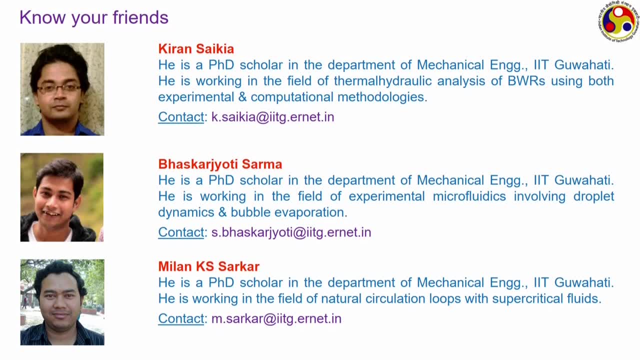 at micro scale, Whereas Mr Milan Sarkar, another senior PhD student. he is working on supercritical boilers or supercritical nuclear reactors, In which, when해 Mr Milansargar, another senior PhD student, is working on supercritical boilers or supercritical nuclear reactors. So 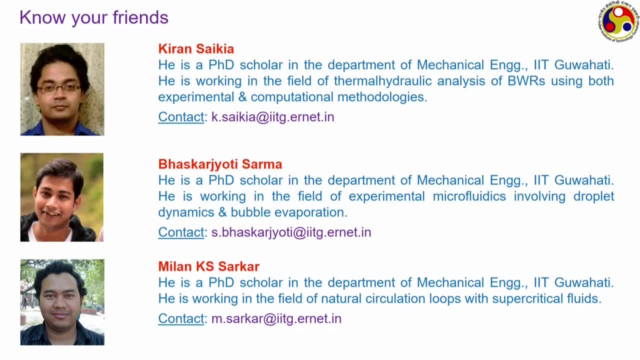 this topic will be topic will take care and when that get done I am going to close some reactors, which is again an advanced level nuclear reactor and, if possible, you would like to mention about that sometimes in this course. Their contact details are also available there so you can send mail to either of them as. 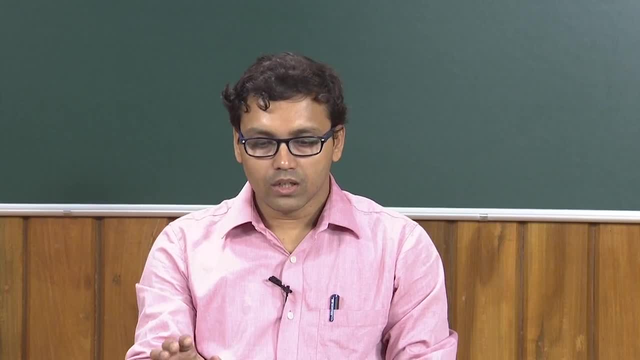 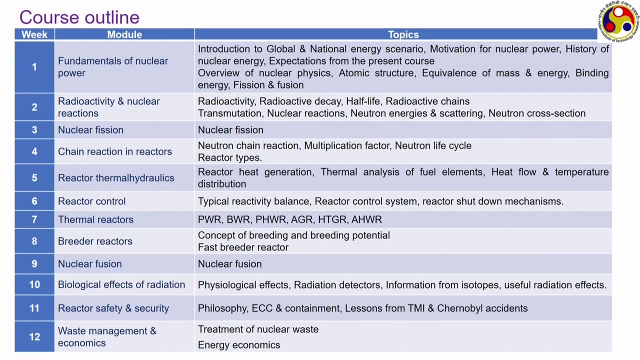 well regarding any kind of clarification. Now it is already available the course outlined on the course web page, but still I would like to repeat here Here this course. we shall be starting from the very fundamentals of nuclear power generation, that is, introducing the concept of atomic power generation, discussing about very briefly 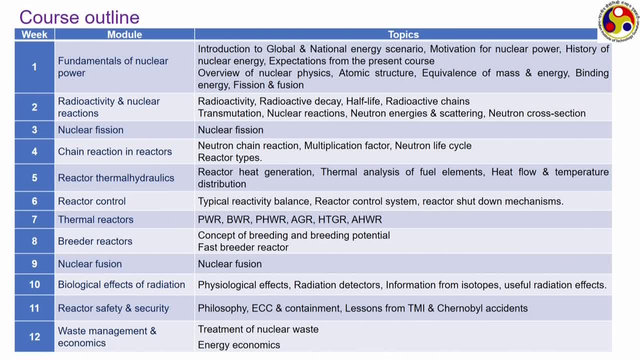 about the atomic structures and the source of nuclear energy, and from there, gradually, we shall be moving to more complicated or more advanced topics. Accordingly, the entire content has been divided into 12 modules and it will span for 12 weeks, So the objective is to cover one module. 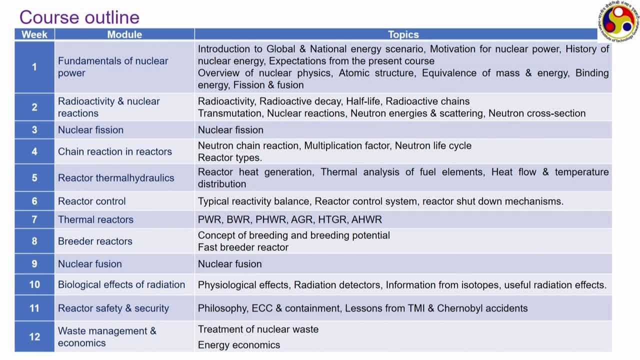 In every week. accordingly, each of the modules- some of the modules, rather, we can be covered in 2 lectures. some of them may require 3 or 4 lectures, and each of the module will be followed by one tutorial. where the tutorial may contain multiple choice, questions may 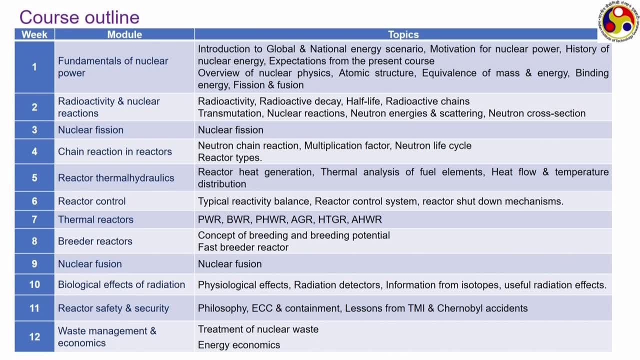 contain numerical problems or may have slightly descriptive one as well, depending upon the content of that particular module. Again, as I mentioned, hint towards the solution of all. the tutorials will be given and we shall begin. I will be there for helping you while solving these tutorials. 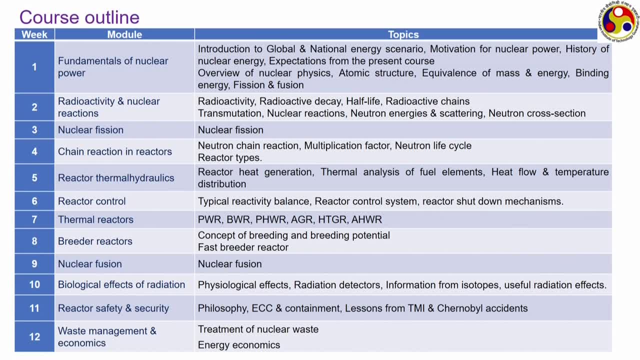 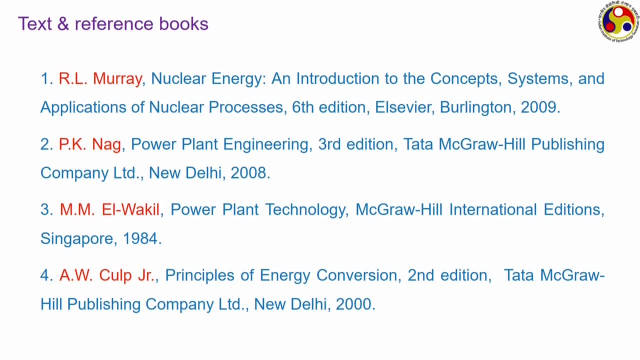 I would also like to solve some sample problems after every module or after any relevant module, And these are the textbooks that we shall be following in this course, where I shall mostly be following the book of Raymond Marais, but many of you may not be having direct access. 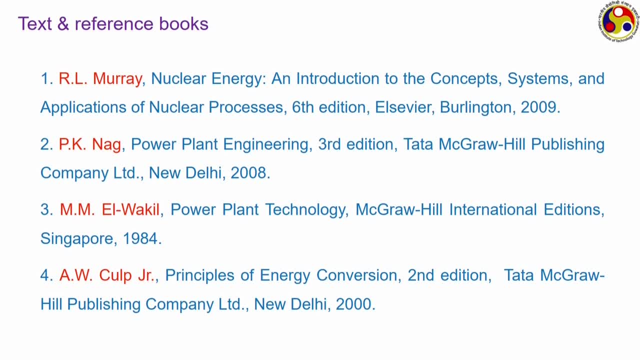 to this one, So you can follow either of the next two: The book on Power Plant Engineering by Professor P K Nag- I think the third edition is the latest one- And also the book by M M L Wakhil on Power Plant Technology, another classical book, both. 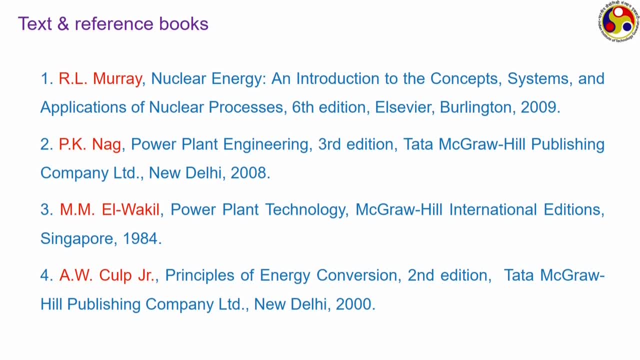 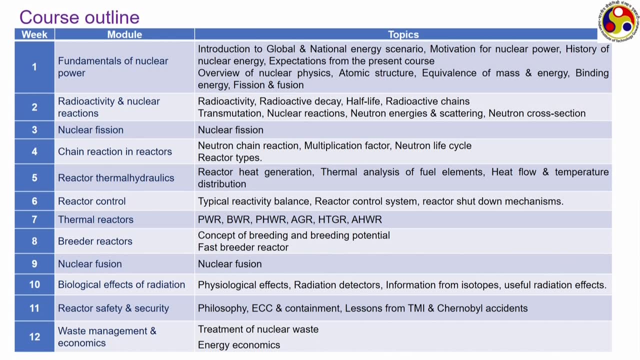 of them has a chapter on nuclear power generation which is very much relevant. And if I go back to the course outline, both of these books will be sufficient to cover up to module number 8 or 9 for this particular course But of course the rest of the 3 modules where we shall be discussing about several advanced 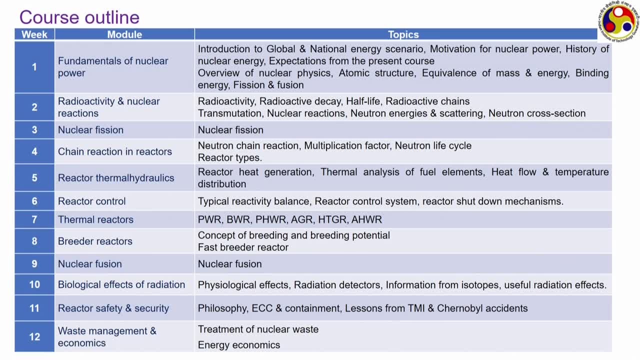 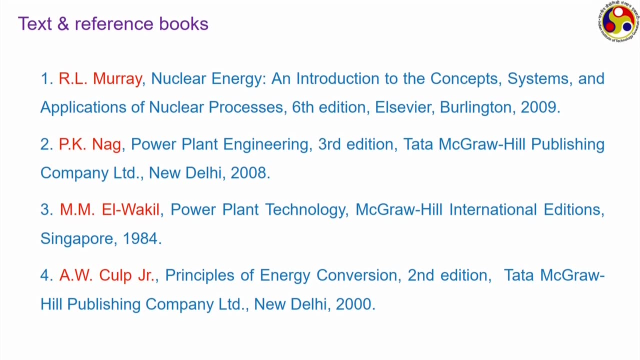 topics such as biological effects of radiation, The reactor safety and security, and also the waste management. these are more modern day topics and they may not be available in the books. you can refer to different materials available on internet and, of course, the lectures will be there for your help. 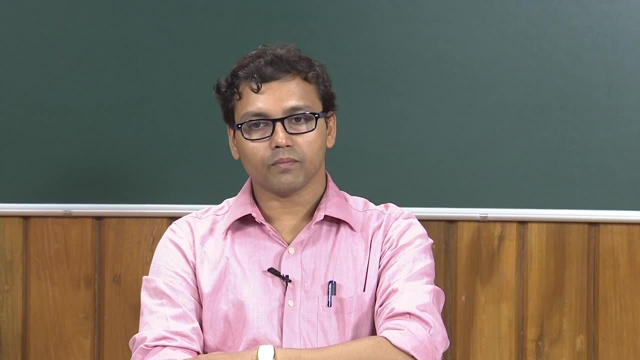 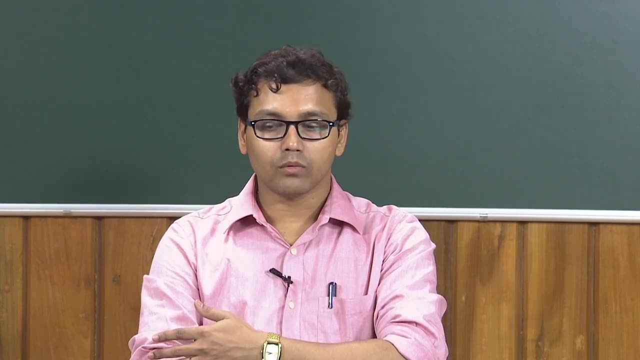 Now the topic of nuclear power generation has a quite rich history. Of course I, in history point of view, I am not talking about the way other sources of power generations were invented and how they came into practice. So I will be talking about that in the next lecture. 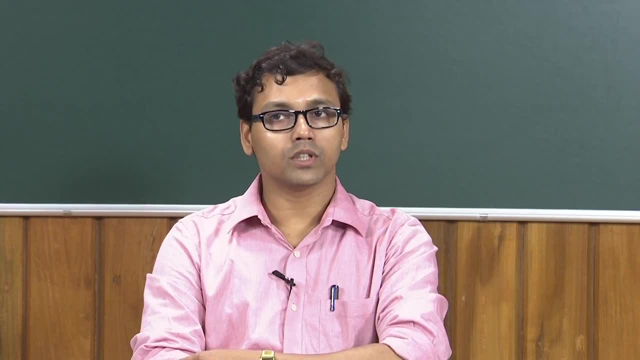 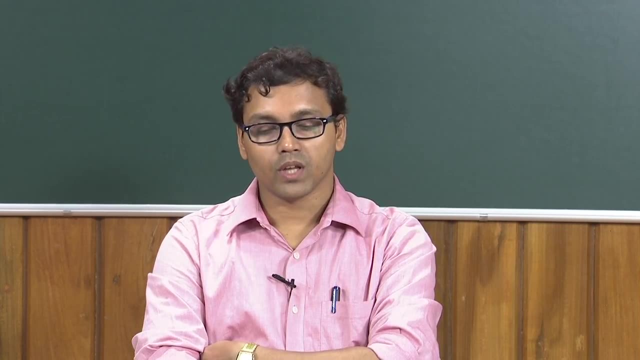 practice. rather it has quite a bit of checkered history, because the term nuclear energy were introduced to the mankind only after that massacre at Hiroshima in 1945. And it is quite fascinating to think that in just about 6-7 decades from that point. 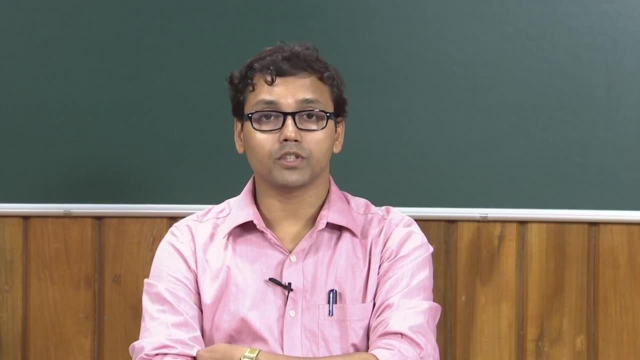 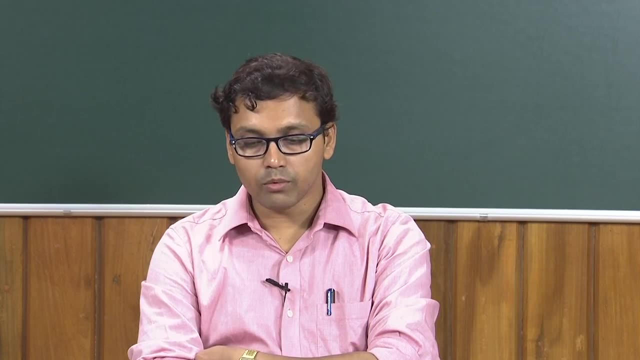 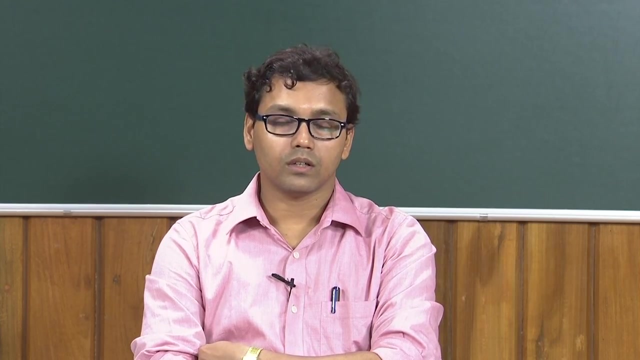 we are discussing about nuclear power as a possible source of power generation or as a possible solution for our future energy demands. Another term which came to the concept of or came to the knowledge of common people as something synonymous to death or destruction. it is only thanks to the contribution of several 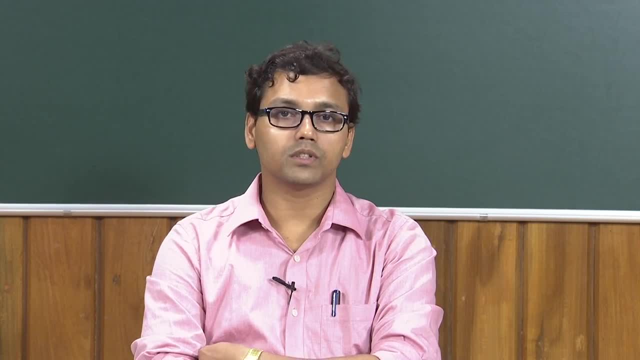 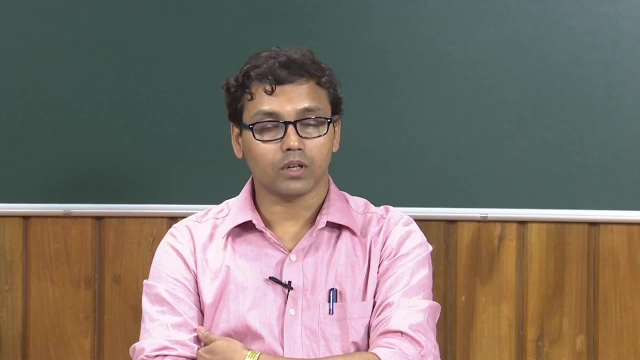 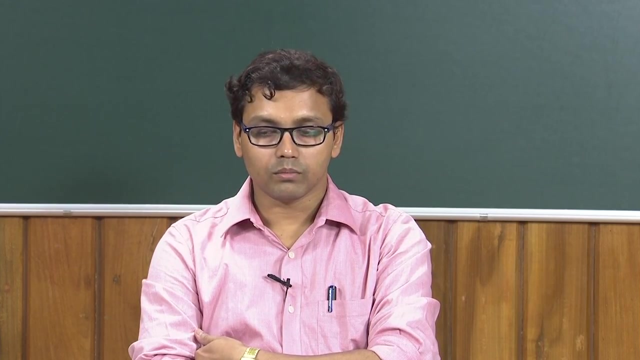 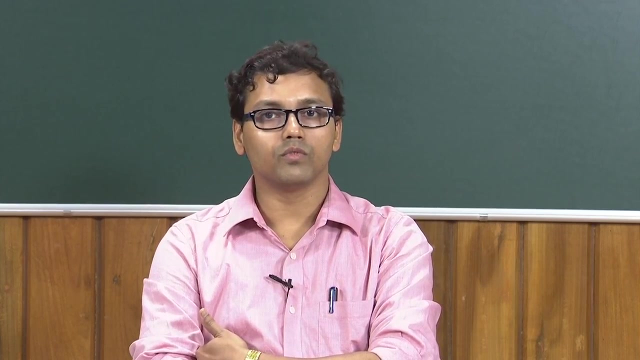 researchers and several scientists who kept on working on this and did not just kept it limited to atomic energy, did not keep limited atomic energy to the weapon related options, rather diverted to the commercial power generation And because of that in only 1950s first commercial nuclear power plant was established and gradually we moved. 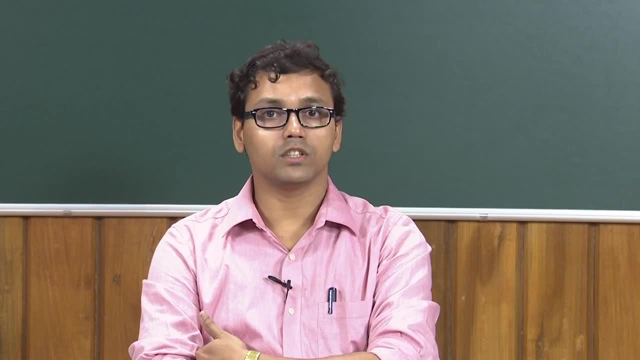 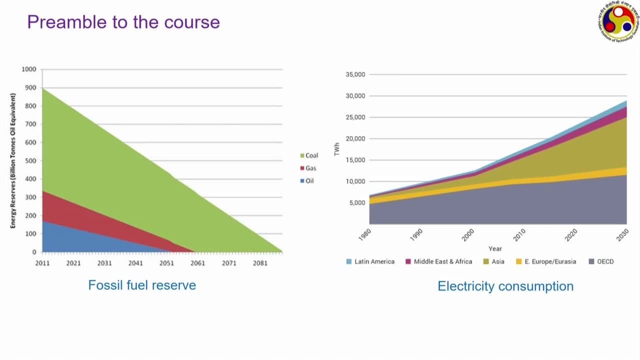 on to get a good share of the global energy production from the nuclear energy. Just to justify the need of knowing the nuclear energy, I would like to show you this couple of projections that I have, This particular one which I am sure all of you are aware that presently we get the energy. 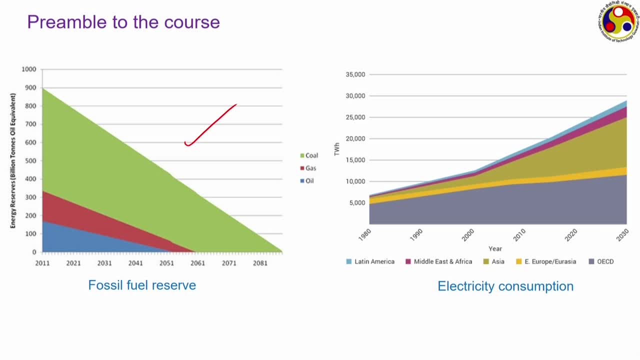 needs. Our day to day energy needs mostly from the fossil phase, like coal, petroleum or natural gases. However, as per considering the present energy reserves available and also the present day consumption, these stocks are not infinite. rather, they are depleting at the very very. 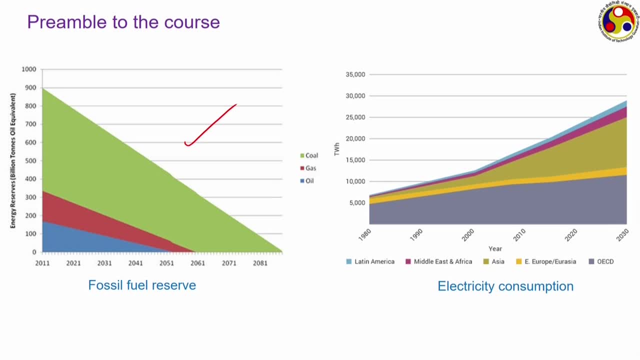 fast rate And just going by this projection, the stock of petroleum and natural gas not expected to last longer than 2050 or 2060, whereas coal may survive for 30, 40 years more, but by the year 2100 we are expected to run dry if we keep on depending solely on this fossil. 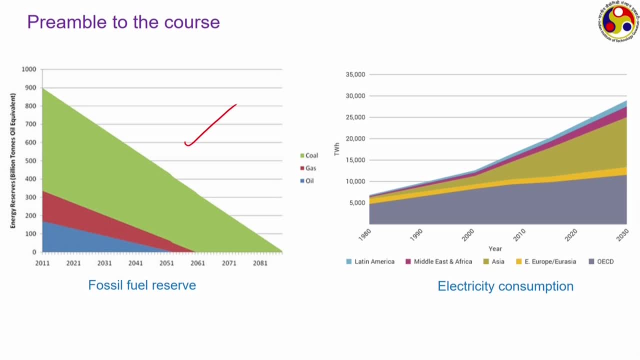 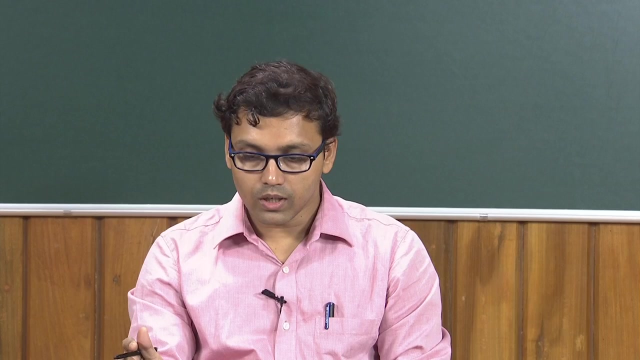 fuels. And now, if we compare that with the other projection, that is where I am showing here the global electricity consumption. you can see here the electricity consumption is not only increasing year by year, but it is actually escalating at a very, very fast rate, Particularly, 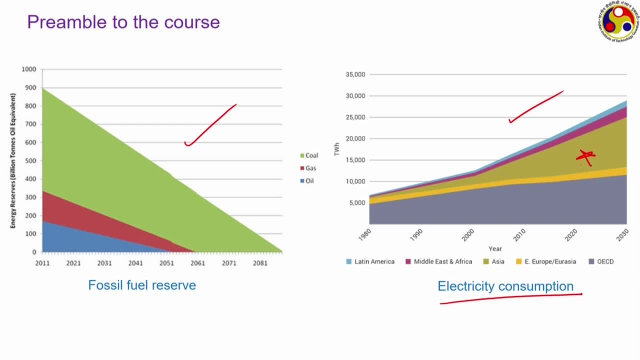 in Asian and Middle East related countries where you can see there is an accelerated growth. If we compare the figures, say from 1990 to 2010,. over this period of 20 years the consumption in the Asian countries has become nearly double, or at least 1.67 times. 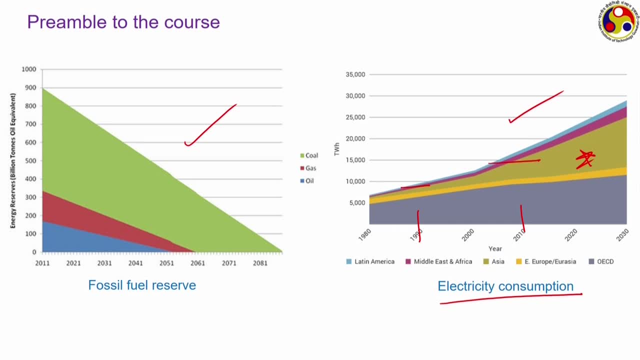 And in terms of the global figure, if you compare this one in 1980, which was 20 years ago, around 6,000 ton watt hour, or tera watt hour we should say- in 2010 it was around 18000.. So a 3 time increase in 30 years And this electricity consumption is only going. 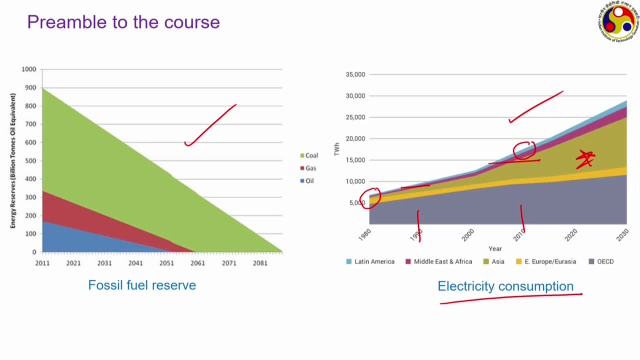 to increase at an even faster rate because of several quite well known reasons, like our fascinations towards electronic gadgets. we are depending on heavier machineries for solving everyday tasks and those sorts of things, And then the electricity consumption is not going to increase at a very fast rate, or at least 1.67 times, we should say, because of 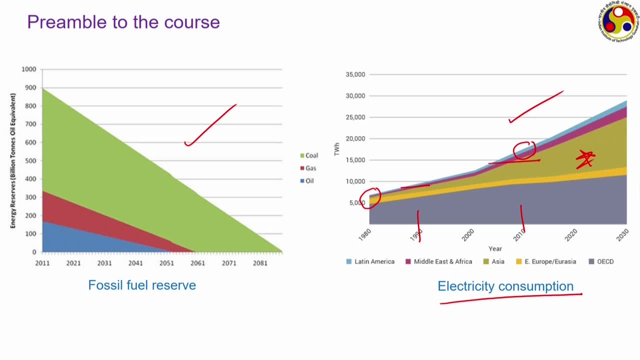 several quite well known reasons, like our fascinations towards electronic gadgets, We are depending day to day needs of ours, our fascination towards illumination and so, and so several reasons, And therefore we need to find some other options without, instead of just continue to depending on the fossil fuels, we have to find some other options of electricity generation. 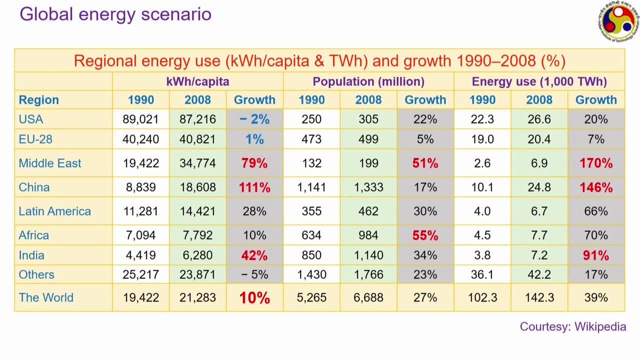 and that is where the renewable and nuclear power comes into the fore. Here I have some numbers to the substantiate the same point. If you compare the figures from 1990 to 2008, you can see the global population has increased by about 27 percent over that period. where in European countries or in some advanced 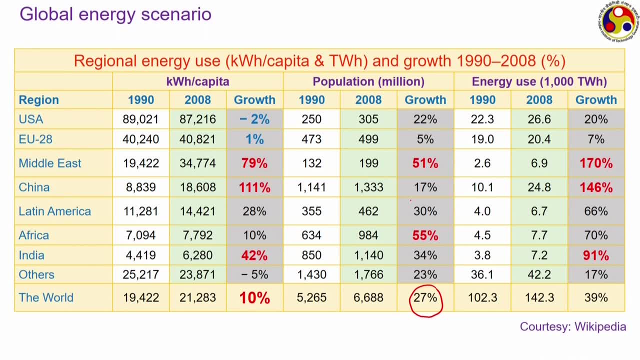 nations the growth rate is quite moderate. China has done quite amicable job because their growth rate is only 17 percent. in Middle Eastern African countries The growth rate is quite high, over 50 percent, and in fact India is also not far behind. 34 percent increase in the population you can see in the period of just 18 years. 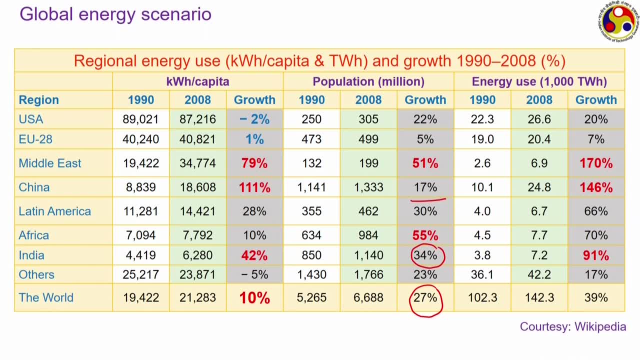 Now, if you compare to the energy users on the last set of data, you can see China has seen 146 percent- a staggering number, really: 146 percent increase in their energy users, while their population growth is only 17 percent. That leads to an 111 percent increase in the population. 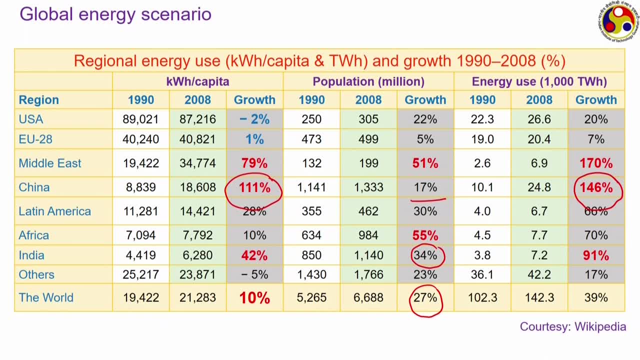 So this is a significant increase In their per capita energy consumption. Middle East is also not far behind. there, the increase in energy consumption is even higher: 170 percent- and so about 80 percent increase in the per capita energy consumption. India has seen the energy consumption becoming nearly double and leading to a 42 percent. 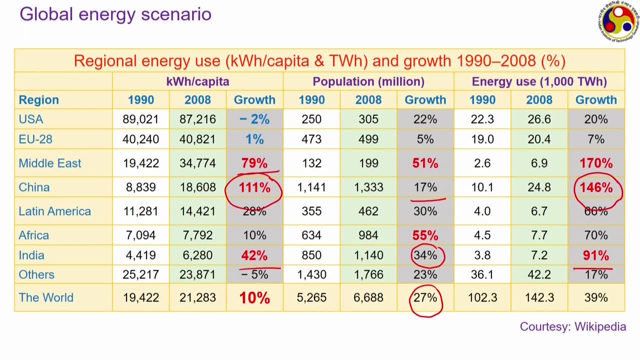 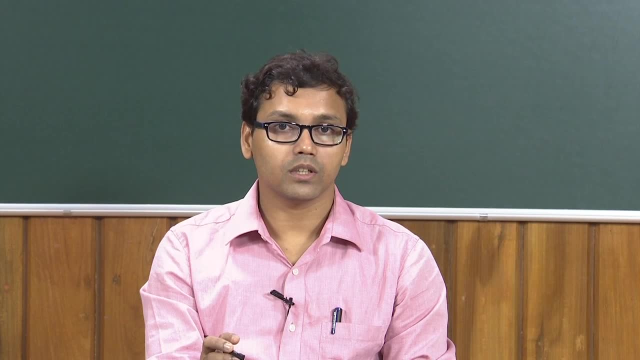 increase in the per capita energy consumption, whereas the advanced countries had done really good job. In addition, in European countries we have seen it to be more or less the same In this others. this involves about countries like Australia and others. here you can see: 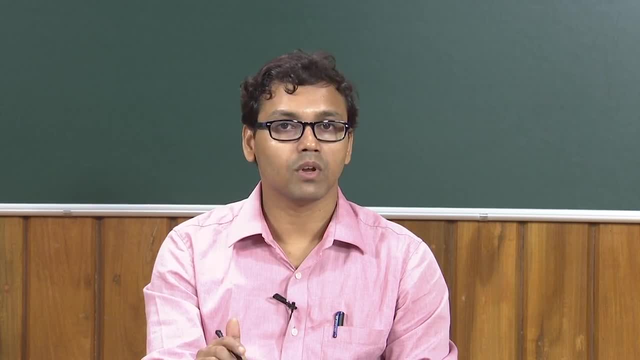 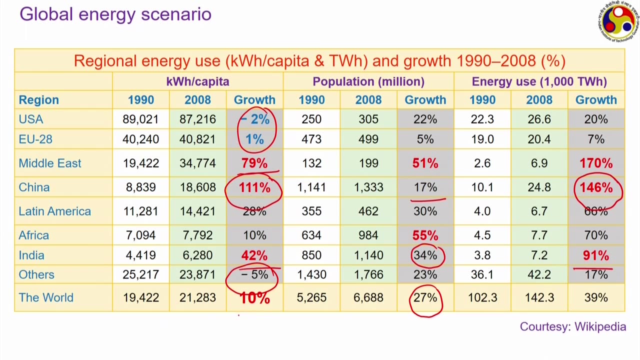 there is, in fact, reduction in the per capita energy consumption, but because of the contribution coming from Asian and Middle East countries, we have more than 10 percent increase in the per capita energy consumption over this period of 18 years. and that figure, that actually 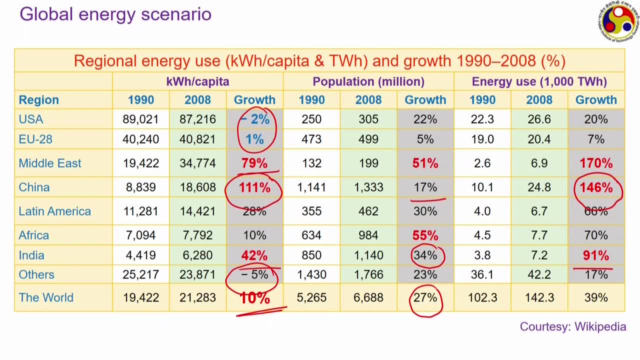 that keeps on increasing And therefore we have to explore some newer option to develop commercial electricity. and that is where the renewable energy and nuclear energy both comes into picture. Now renewable while conventional renewable sources like solar, wind, biomass. they definitely have a great future. 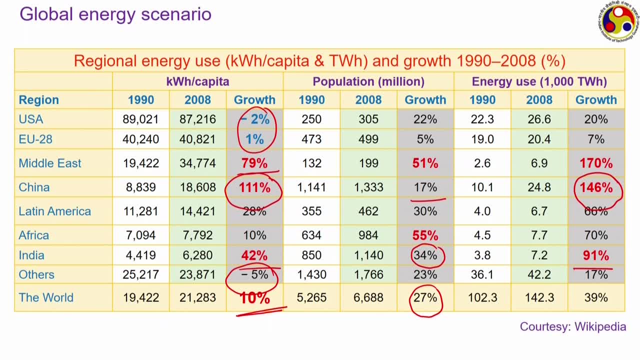 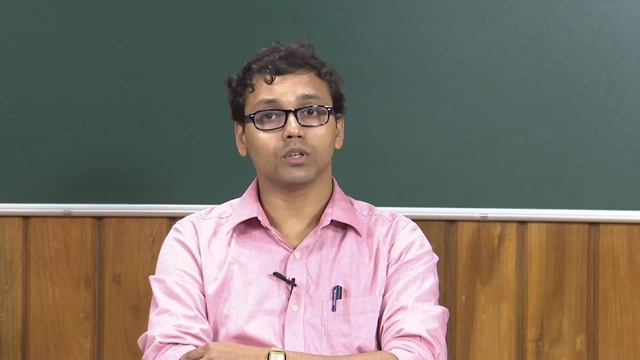 There are several issues as well, particularly their intermittent nature. like you know, solar energy can supply electricity only during the daytime and not at night periods or periods of zero or insufficient solar insulation. wind energy requires a particular wind velocity and so they are very much location specific, somewhat similar about biomass. 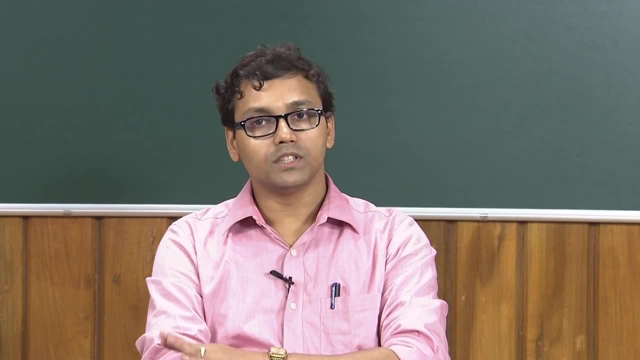 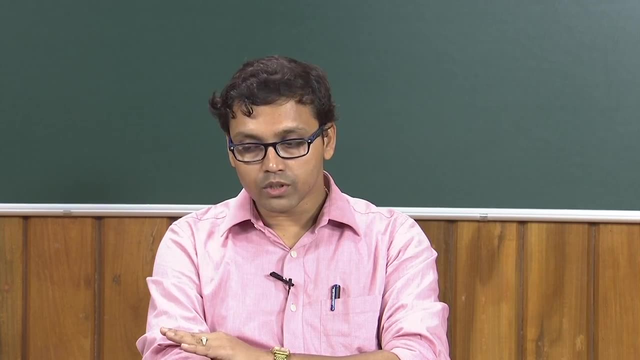 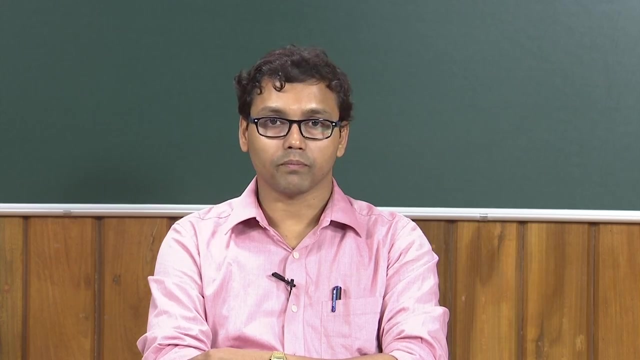 And because of all these factors, the renewable energy till date are restricted more towards local scale, or they are more being thought about peak load stations, that is, to meet the demand during the periods of the highest consumption. Of course, effort is on to have base load solar or wind power stations, and they are 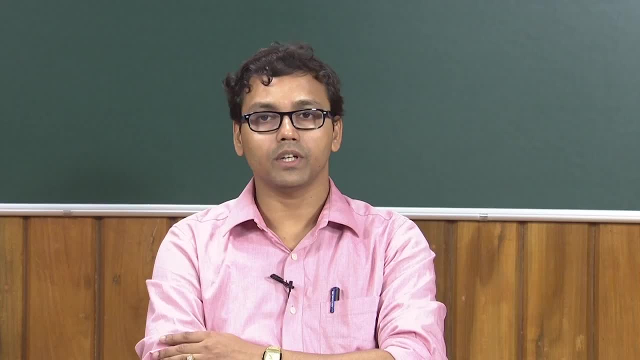 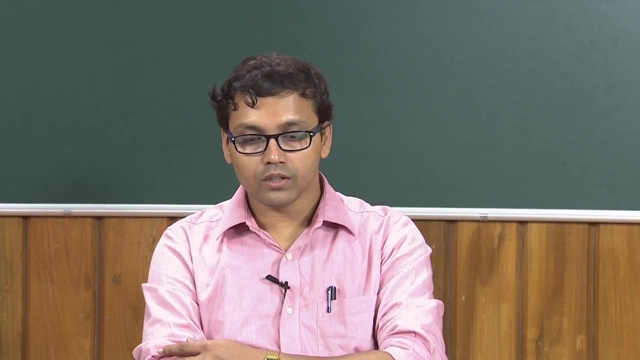 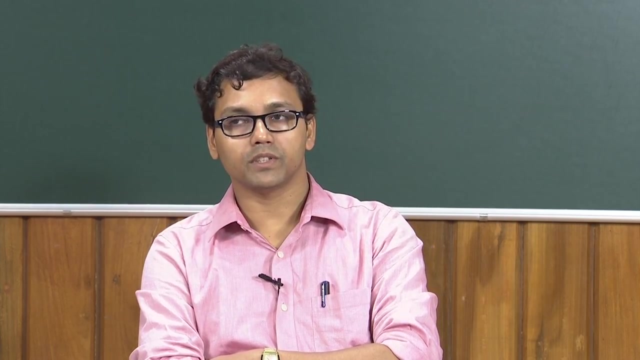 coming, even coming up in different countries at a different rate, and that is only going to increase in future. But there are still several issues to solve, like in: whenever you talk about nuclear, even without knowing anything, people always keeps on complaining about the possible effects on the environment, etcetera. 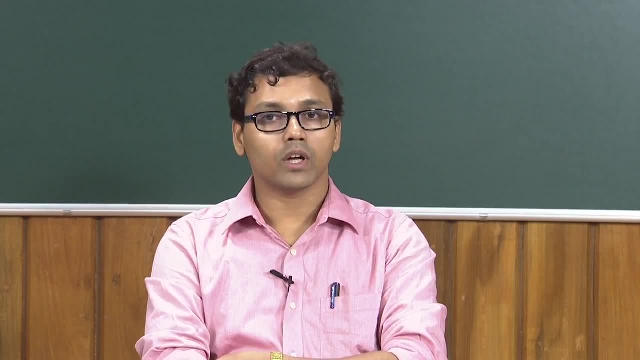 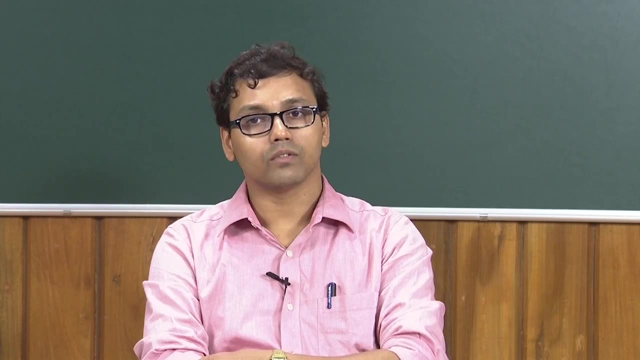 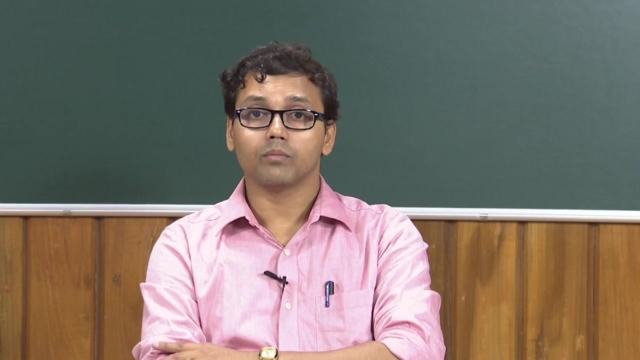 But the conventional power sources like coal and hydro can have as detrimental impact on the environmental effect as nuclear. wind has huge reservation from environmental protection point of view. the installation of wind powers, in fact, And that is where nuclear, particularly about that point- on base peak load station nuclear. 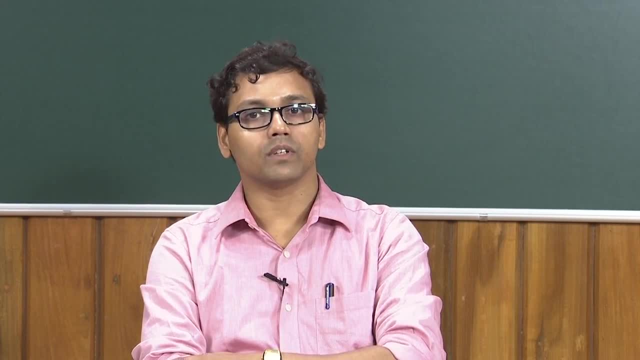 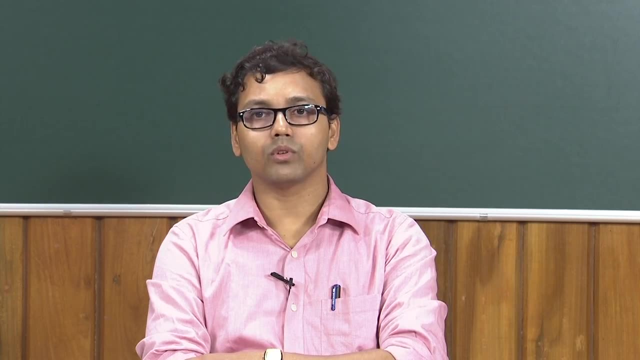 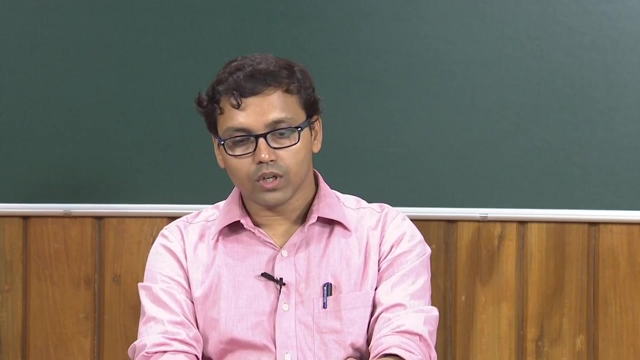 scores higher than renewable, because it can act as a base load station. it can supply a continuous amount of electricity throughout the year without being bothered about the surrounding or environment or any other demographic issue. So that is the point, Thank you, And therefore we also need to focus on nuclear. 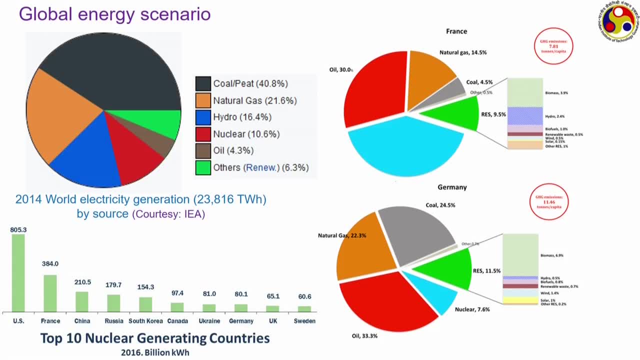 And that is why, if you see the global energy scenario- I have the data of 2014 here- Nuclear steel is a quite small fraction, only 10 percent of the global energy consumption, but this percentage is actually increasing, despite protection, despite reservations from. 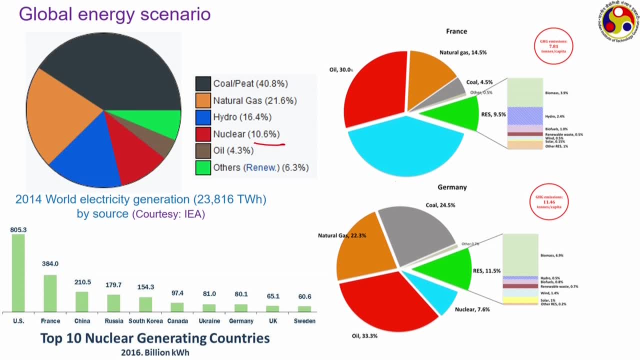 different sectors, The nuclear energy is there to exist. If we see the country-wise scenario, USA is the largest contributor. In fact, if you see this figure, this number, that is, production from US, nuclear energy produced from US in the year 2016, is more than combining the next three. that is, France. 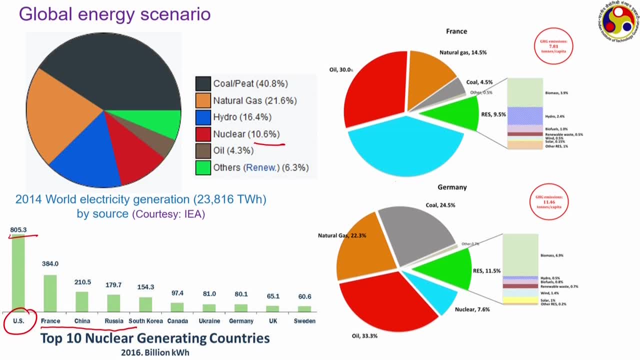 China and Russia, But US is a huge country and that requires very large amount of electricity. So, despite such large numbers, actually nuclear energy is a is a large amount of electricity, So that is why this figure is important. So nuclear energy is produced from USA in the year 2016.. 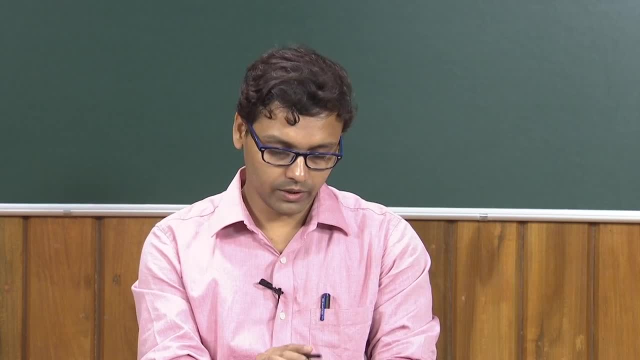 But this has an impact on energy production as well. Then we will talk about the situation in the coming two years And then, last but not the least, the next three years we will talk about. that is why nuclear quite small portion of the total energy produced in US. 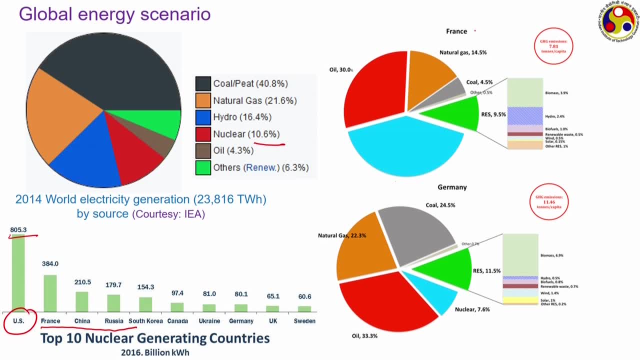 But there are certain countries like France. France gets a good share of their total energy from nuclear. If you see this figure, nuclear contains a very large fraction in this particular case, which is well above 45 percent in France, The principal reason being the absence of fossil fuel sources in France, like their coal. 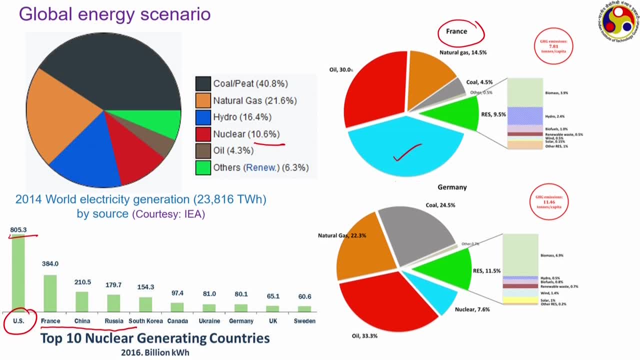 or oil reserve are quite limited compared to other countries. Just compare that to that with their neighbor, Germany. Germany has a very decent reserve of coal, and that is why they are getting much larger fraction of their energy from coal, which is just about 4.5 percent. 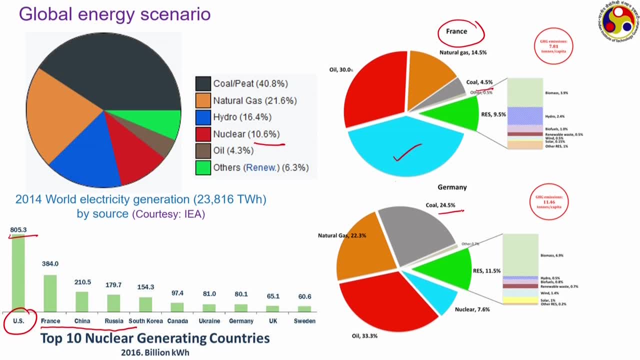 In France it is 24.5 percent in case of Germany, and their nuclear share is quite small. But I would like to To attract your attention to another figure. see the greenhouse gas emission in case of France was 7.81, whereas that for Germany is 11.46.. 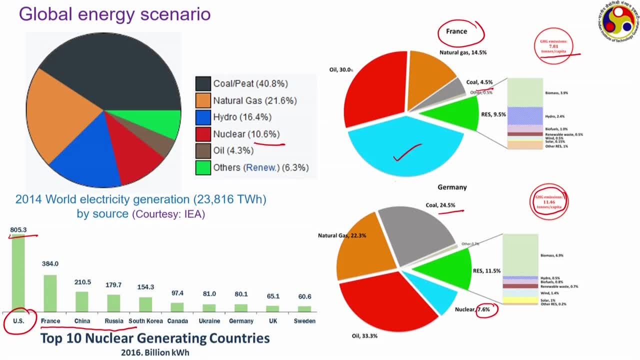 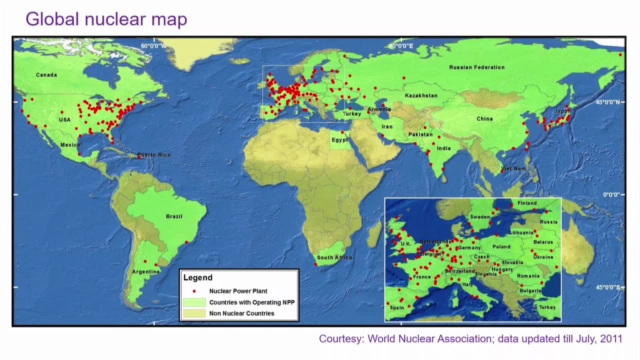 I shall be coming back to this figure after a few slides. This is a global energy map- slightly old data- of 2011.. You can see in Europe and US- in European countries and US- there is a good spread of nuclear energy, And also in Japan. Japan is a country that depends a lot on nuclear energy, despite that. 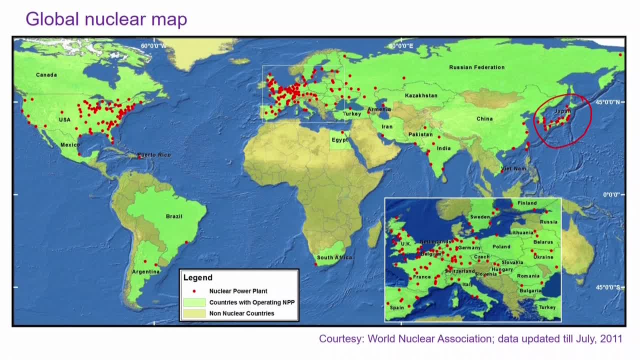 Fukushima and associated effects. India and China has seen an increase in their total nuclear production over last one of two decades And therefore of course there are other areas, like in Africa or in Latin America there are very, very few nuclear energy sources, Or in the eastern part of Africa. 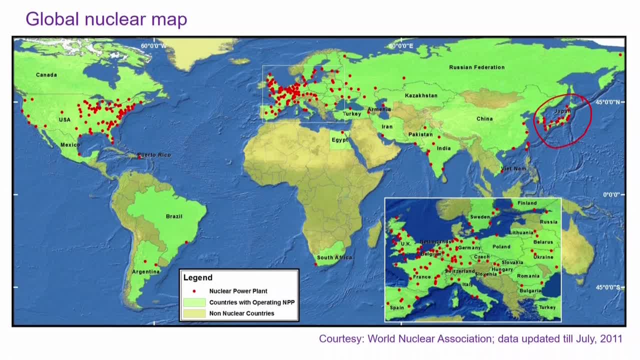 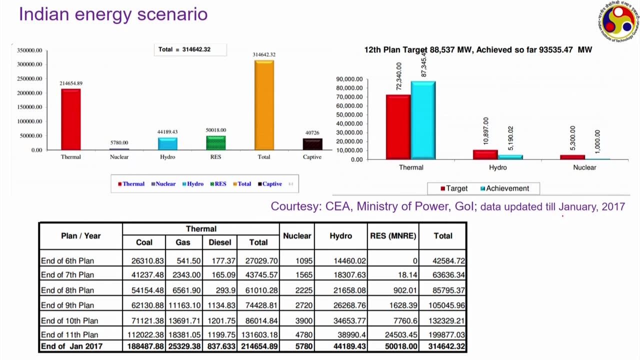 So there are very few nuclear energy sources- And also in Japan- Japan is a country that depends a lot on nuclear energy- And also in Russia, But the feasible reason being the absence of corresponding uranium or other kind of fuels. Now, coming to the Indian scenario, by the year 2017, January 2017, in fact, India was 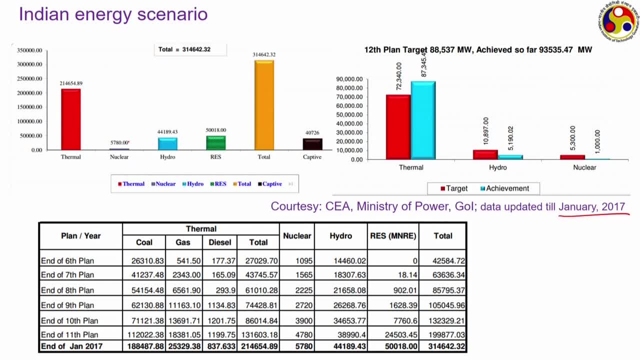 getting only a small fraction of their total production from nuclear: just 5780.. If you compare that coming from thermal it is extremely small fraction. But from what that that? I would like to again draw your attention to this next figures, where I have shown an. 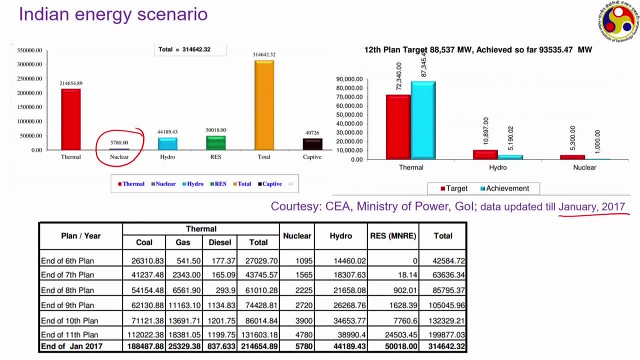 year wise, or the increase in the consumption from different sources, increase in the production from different sources over different 5 year plans, And now, if you see the numbers at the end of the 11th plan and also till January 2017, the increase in nuclear, while it is only about 1000 megawatt, actually magnitude wise it. 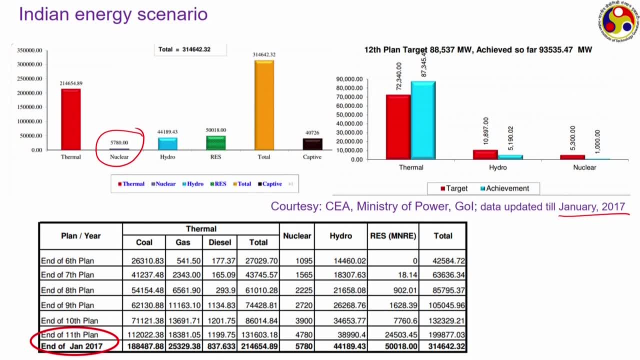 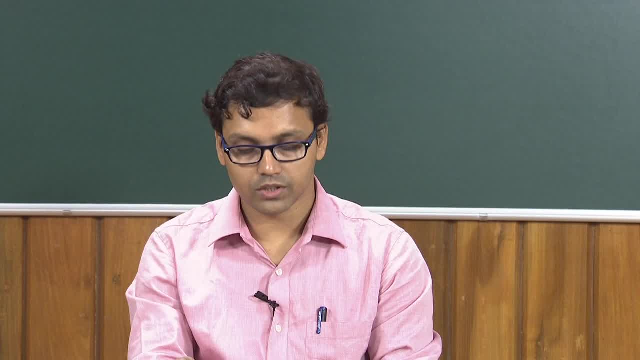 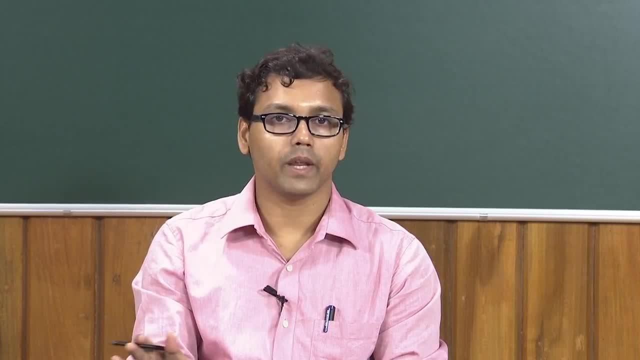 is quite small compared to others. But now, if we compare that from percentage, over this period hydro energy production has seen only an 11 percent increase, whereas nuclear energy has seen 21 percent increase And as there are several nuclear power plants are planned in India, it is expected to increase. even more. In fact, this 21 percent has gone even further because this data is till January 2017.. But the latest Indian nuclear power plant went operational in March 2017, which added another 1000 megawatt capacity to this. 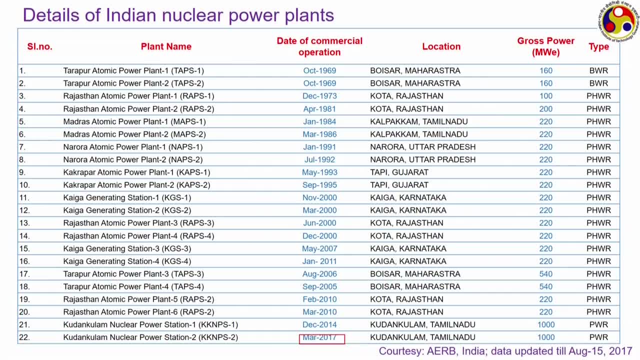 And these are the break up of Indian nuclear power plant, started in as old as 1969, from that Tarapore atomic power plant And that kept on increasing at a faster rate. And these are the break up of Indian nuclear power plant, started in as old as 1969, from that Tarapore atomic power plant and that kept on increasing at a faster rate. 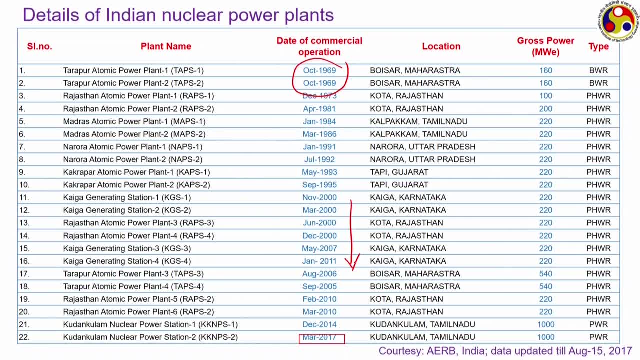 Particularly seen 2000 onwards, you can see there are several plants coming on And the last one, as I have mentioned, in March 2017, another 1000 megawatt capacity was added, which gives a total 6780 megawatt electrical of installed capacity of nuclear power plant. 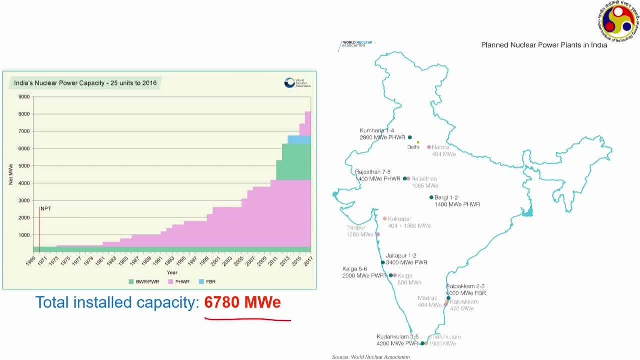 in India And there are several other plants proposed, like. the map here shows quite a few such locations And by 2020, there are several other plants which are expected to becoming operational, Giving or giving a projected generation capacity of 8000 megawatt electrical, or actually slightly. 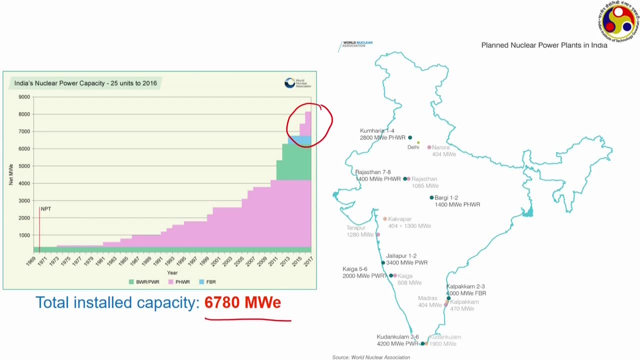 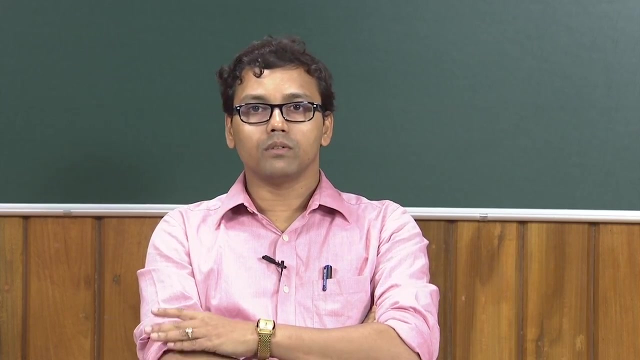 more than that. Therefore, nuclear energy is here to stay, And hence we need to have a detailed idea about this Now. you must be aware that whenever there is a talk of setting up a new nuclear power plant, there will be lots and lots of deliberations and discussions and arguments compared to any conventional power stations. I personally feel that most of that can be ascribed to the lack of knowledge about the technology. People are not properly aware about exactly how this technology works, exactly how energy is harnessed from the atoms, exactly how we use the fuel or how we can protect the surrounding. 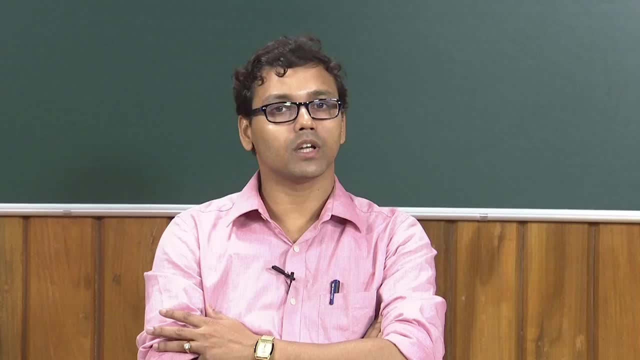 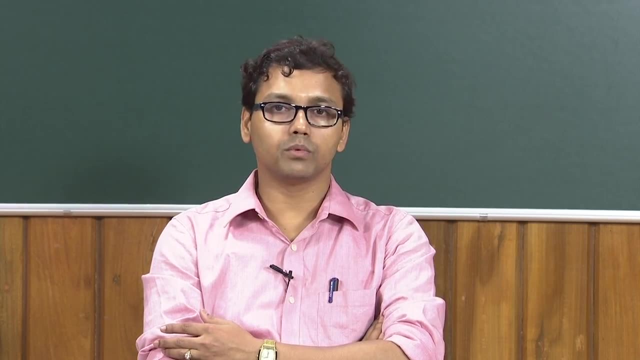 from radiation hazards. exactly what are the nature of this radiation hazards that we always keep on discussing? How we discard the spending energy, How we drain fuel or how we dispose the waste fuel? If we have proper knowledge about them, then probably we shall be in a much better position. 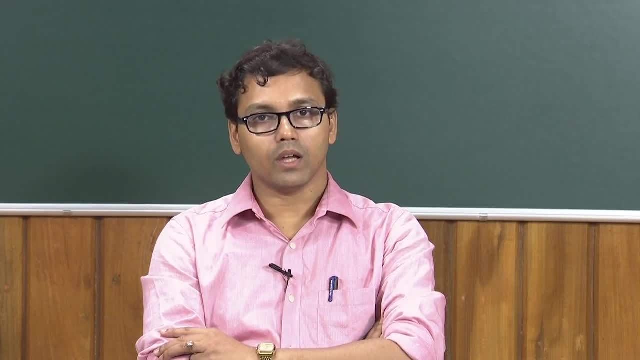 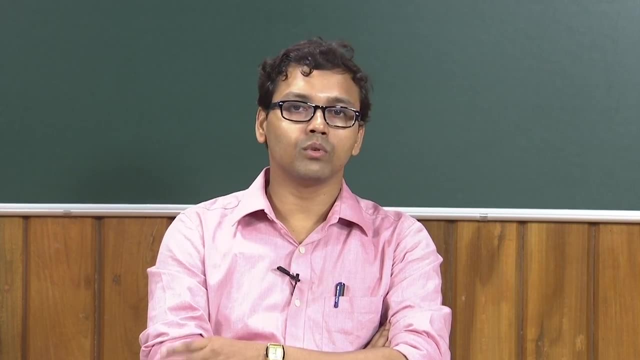 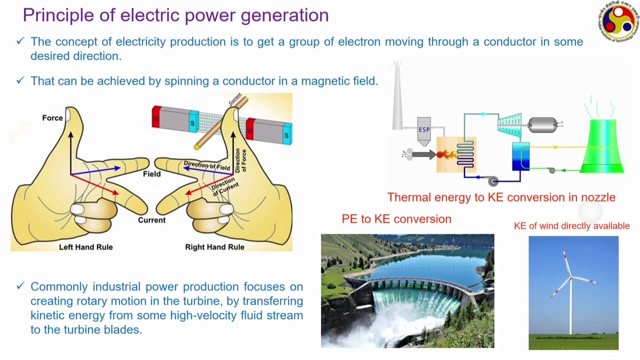 to discuss whether we should go for nuclear energy or not, And I am sure that successful completion of this course will allow you to participate in those discussions and put on your own points for this. So let us start with very basic principle. We shall not be discussing too much about the nuclear power generation as a topic, rather, 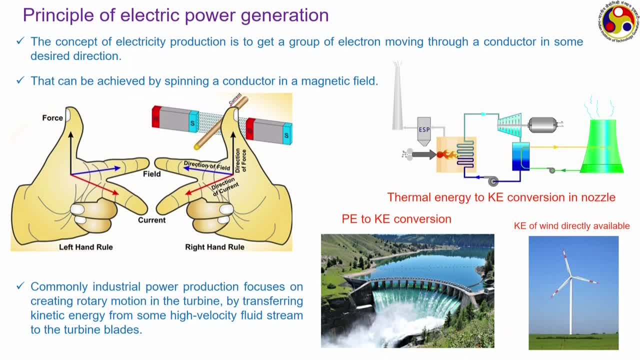 we shall be discussing more about some introductory points about how energy is produced. what are the top points where nuclear is separated from the conventional sources, what are the advantages and disadvantages of nuclear energy? And also we like to plunge very briefly into the history, paying our homage to several great 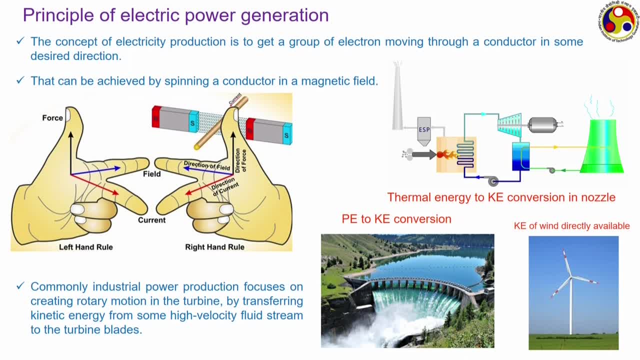 minds who have contributed to the development of this particular technology. And finally, we shall be look into the atomic structure so that we can prepare ourselves to go more in depth discussion on the nuclear generation. So now, here we have the principle of electrical power generation, which I am sure all of you 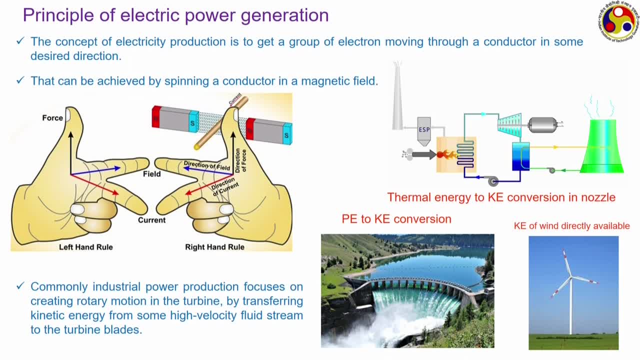 are aware about The electricity production is achieved when a group of electron is able to move through a conductor by some at some desired direction, and that movement of electron is generally achieved By spinning a conductor in a magnetic field. Now, up to that part more or less all power stations or conventional power stations have 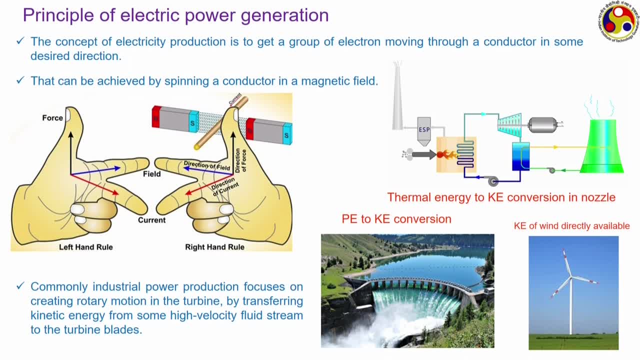 the same kind of working principle, But how to create this motion of the conductor. there is a difference. In most of the common power stations you will find a turbine which has several blades mounted on it and the turbine itself is mounted on a shaft. We create the rotary motion of the turbine by heating the turbine blades with some high 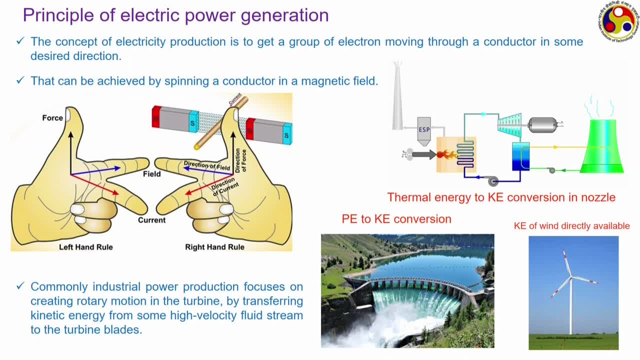 velocity fluid stream, So that the kinetic energy of the fluid stream is transferred to the blades and subsequently to the shaft, and alternator is mounted on the same shaft, which gives us the electricity as the output. Now, the difference between different kinds of power stations is the way of producing. 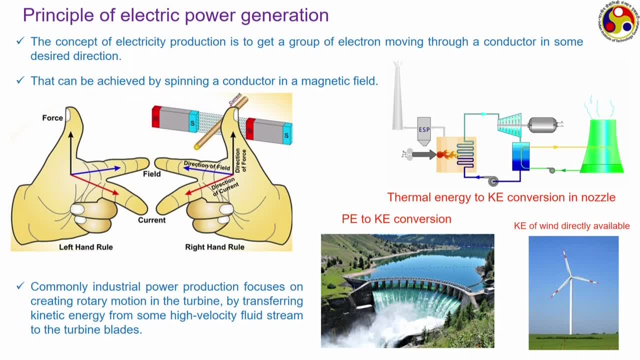 that high velocity fluid stream. Like in case of a coal based thermal power plant, we have thermal energy to kinetic energy conversion in the nozzle, Basically coal or such kind of fuel like coal. So we have thermal energy to kinetic energy conversion in the nozzle. 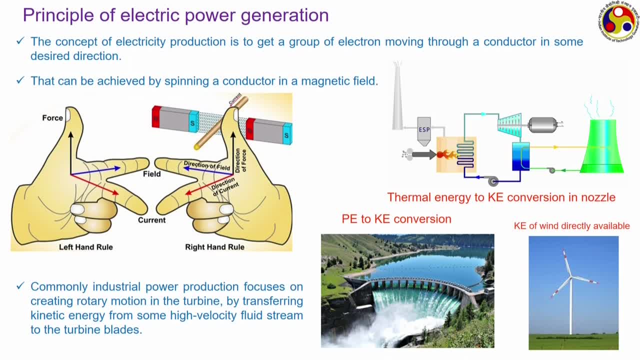 Basically coal or such kind of fuel like coal. So we have thermal energy to kinetic energy conversion in the nozzle. So we have thermal energy to kinetic energy conversion in the nozzle. So we have thermal energy to kinetic energy conversion in the nozzle. 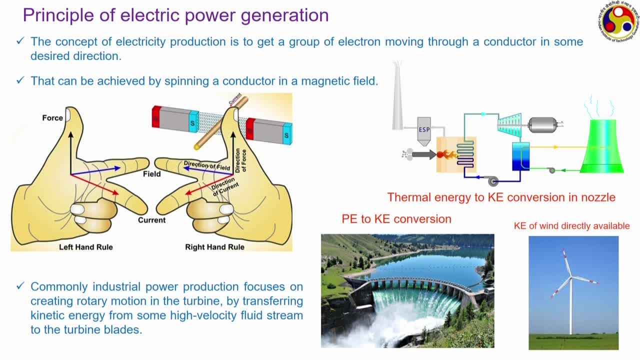 Like any gas, etcetera, is burnt in the boiler So that the heat of combustion is used to generate steam. by supplying that to water we get a high energy or high enthalpy stream of steam that is taken through nozzle and it passes through the nozzle that thermal energy is converted to kinetic energy, which 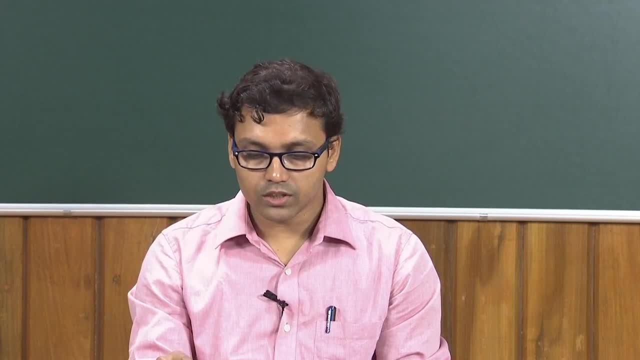 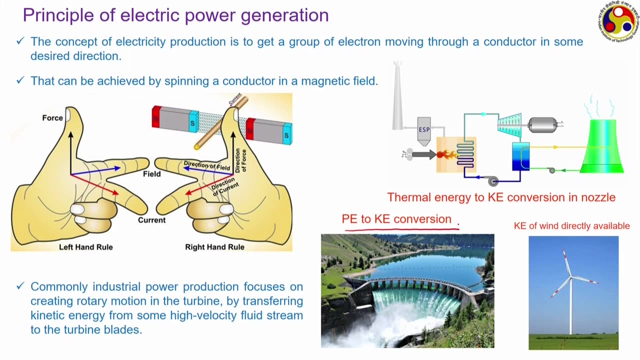 is subsequently taken to the turbine, Whereas in case of hydroelectric power stations- here we know that water from a higher, from a higher current is generated- elevation is allowed to fall through, thereby converting its potential energy to the kinetic energy. and when this high velocity water jet strikes the blades of the hydraulic turbine, 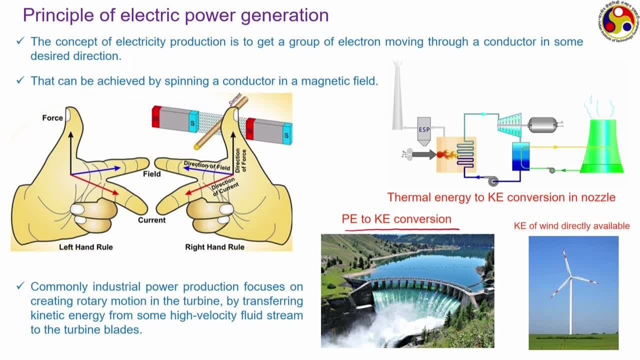 then rest is the same. And this kinetic energy is readily available in case of wind turbine, because we need a certain velocity of wind, so which will be able to move the turbine blades by a certain magnitude and certain rpm rather, and that will subsequently lead to the production of 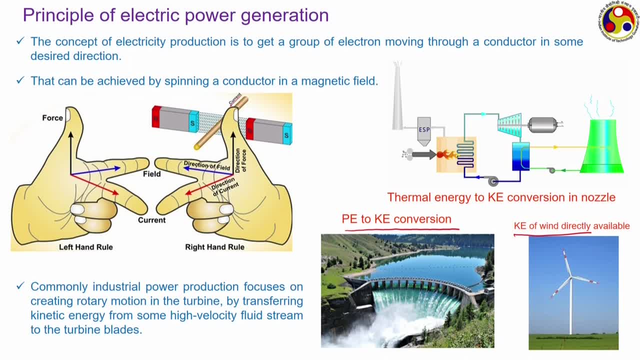 electricity. Now there can be two types of this: high stream energy or high velocity energy generation we can divide in two categories: One, like this hydro or wind, where we either directly get the kinetic energy or convert potential energy into kinetic energy. The other where thermal energy involved, like coal. 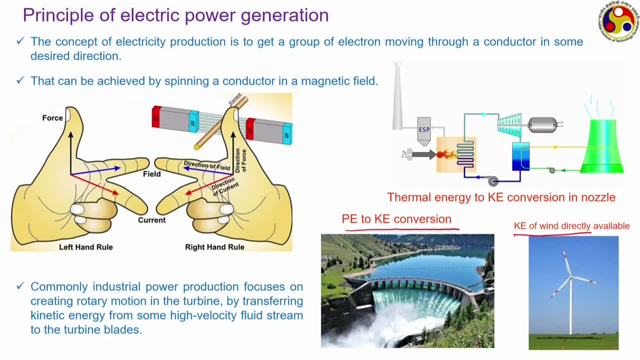 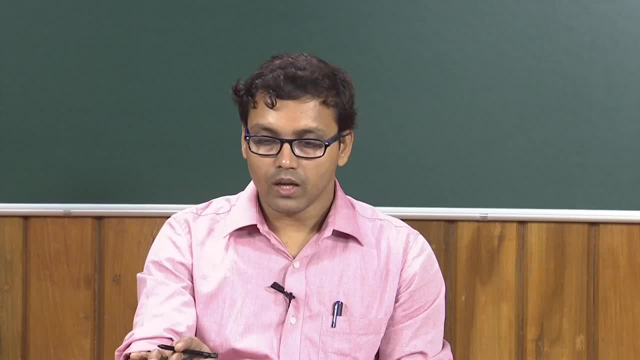 Where we generate. We generate thermal energy by burning some fuel or by some other means, and that thermal energy is used to raise steam and then rest through the nozzle and the turbine. And nuclear is in this latter category, that is, it is quite similar to the coal based power. 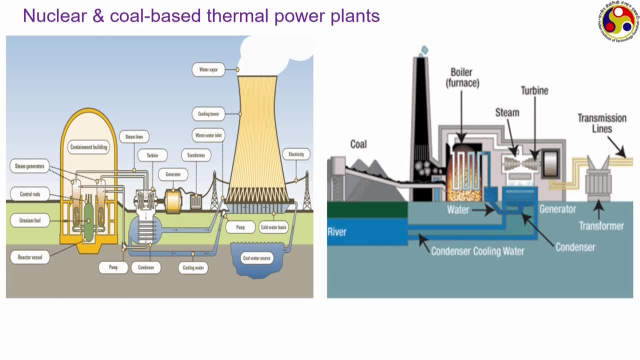 stations. In both the cases, several components are same. like you will be having the same kind of nozzles and turbines, a steam generator where energy is supplied from some fuel to produce steam. Then you may have a condenser, boiler, feed pumps and all those associated accessories. 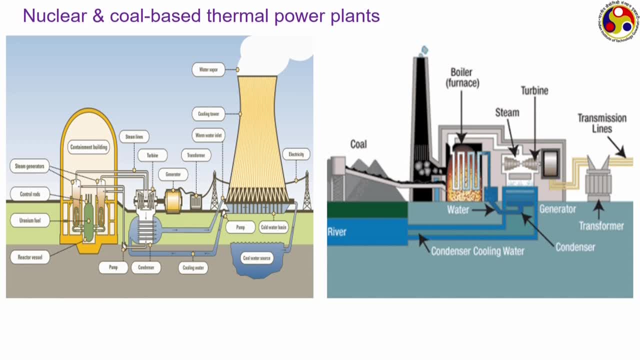 But their difference is how we supply the energy to the steam. in that steam generator, Like in case of coal based power stations, we have chemical energy of fuel converted to the thermal energy. Now there we have basically a chemical reaction, and any chemical reaction means rearrangement. 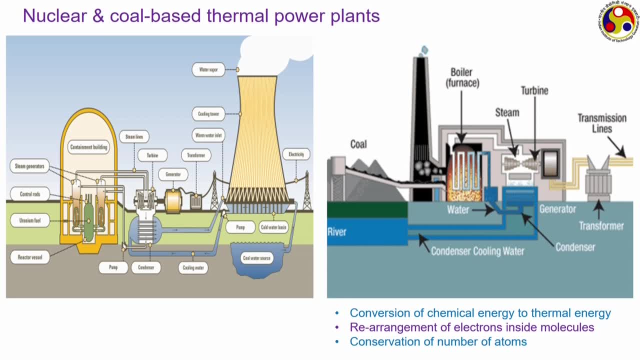 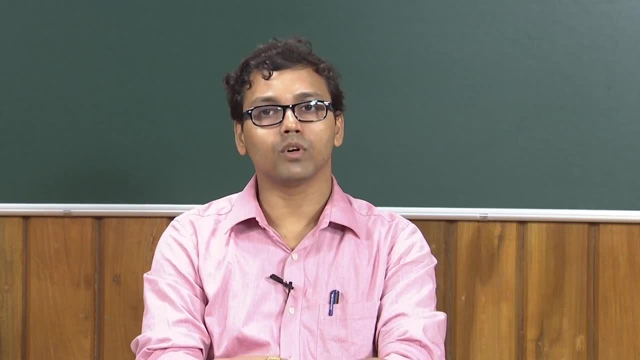 of electrons inside the molecules So that we can generate thermal energy. So we can generate thermal energy Now, the number of atoms are conserved, but atoms combine in different way to form different kinds of molecules. So the total number of molecules may not be conserved, but total number of atoms and electrons. 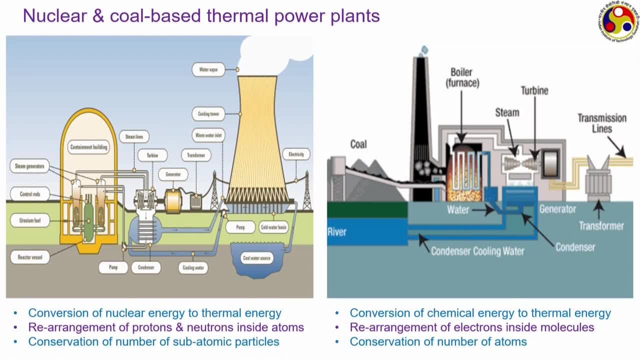 will be conserved. But in case of a nuclear, we have conversion of nuclear energy to the thermal energy, where not electrons or we are not at all talking about atoms or molecules. rather we are going inside the atoms and we are into the nucleus where the protons and neutrons they will be. 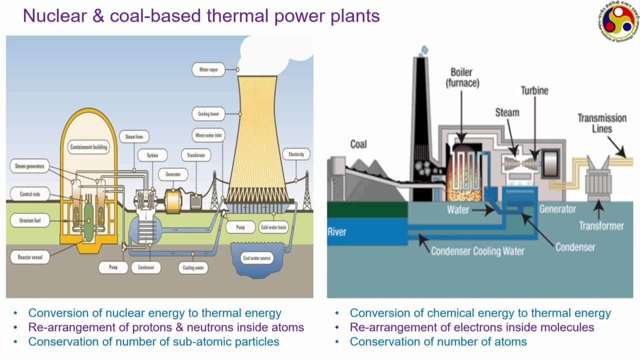 rearranged. They get arranged to form a new nucleus, giving birth to a new atom, And therefore total number of the subatomic particles, that is, protons and neutrons, will be conserved, but total number of atoms may not be conserved. we shall be discussing about. 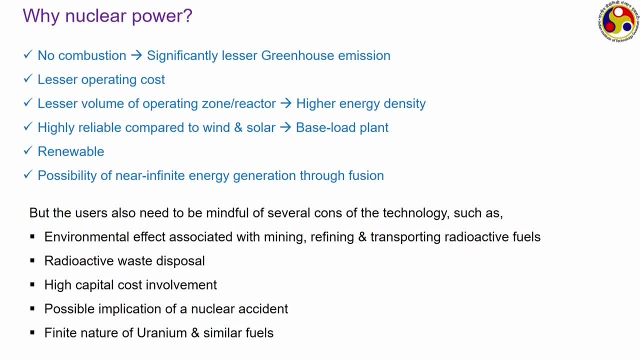 this in more detail. Then I have to justify why should we go for nuclear power. and here I have jotted out a few points. Some of those will be discussed in more detail later on. The first one is no combustion, Of course. i have seen that if you want to get rid of the carbon from a nuclear plant, 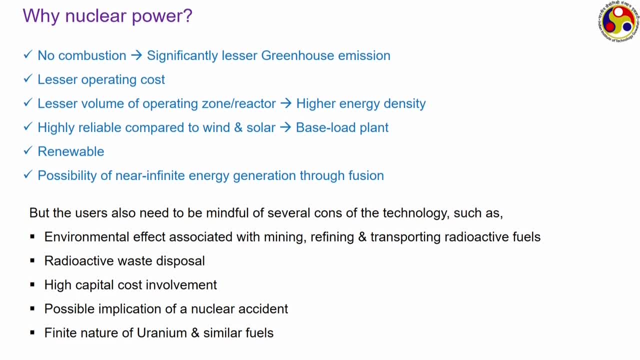 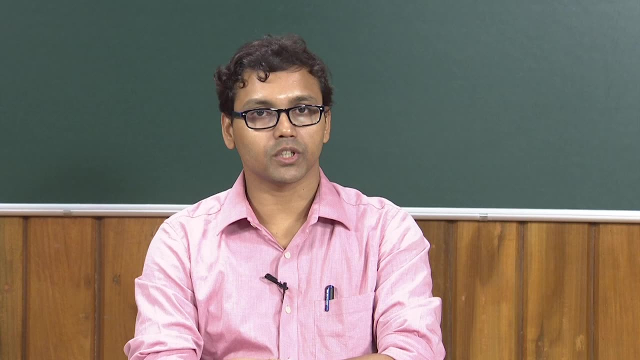 Then you should take out a Afghan particle from a nuclear plant. Of course, in case of coal based power stations, we burn the fuel and exhaust gases are allowed to escape to the surrounding, leading to environmental pollution. and such kind of greenhouse emission is absent in case of nuclear because there is no chemical reaction involved. 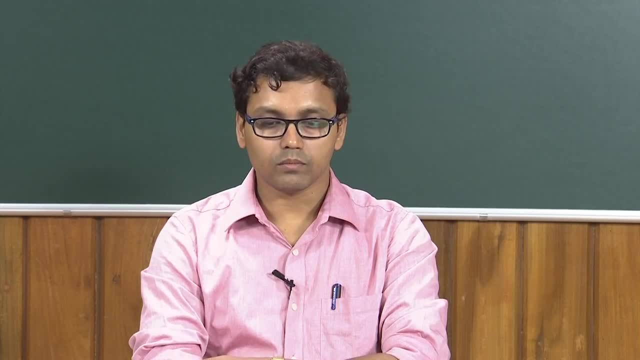 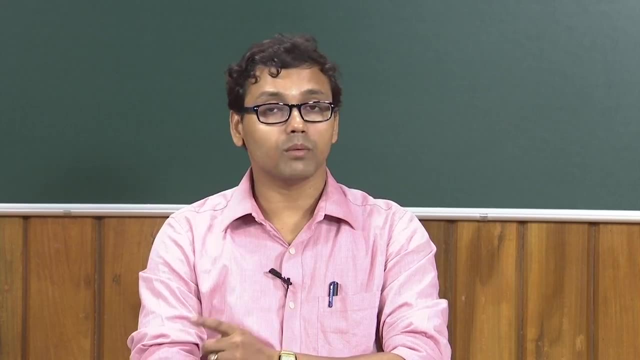 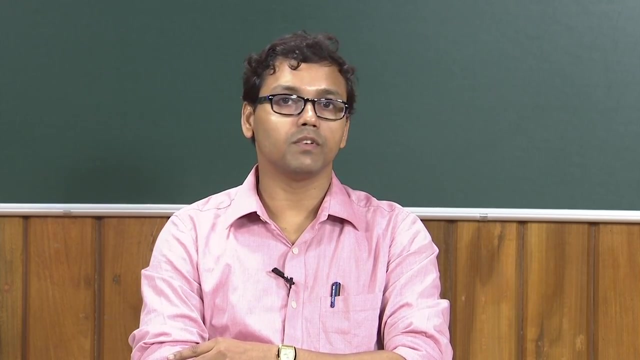 Whatever happens, that is happening at the atomic level only, and greenhouse emission will therefore be subsequently significantly lesser. I have shown you couple of numbers for France and Germany earlier. if you remember, in case of Germany, the amount of greenhouse gas emission was at least 50% more compared to France and one primary reason being this: because Germany depends a lot on coal based power stations or power generation and similarly oil based, that is, combustion related technologies, whereas France gets a significant share from nuclear. So nuclear definitely is a much cleaner technology compared to coal. The operating cost: 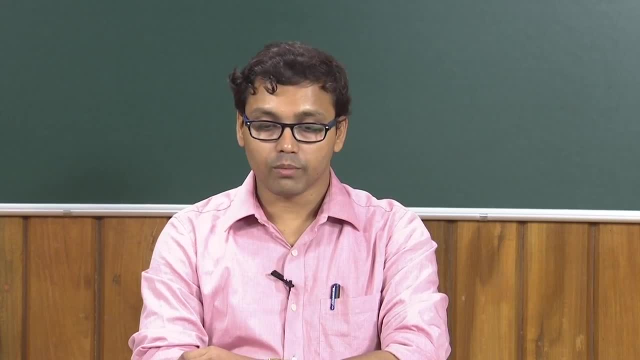 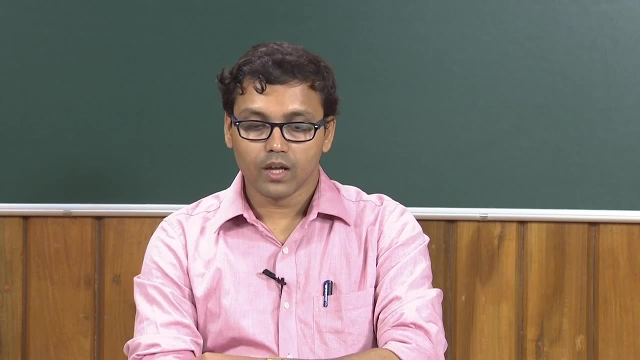 The operating cost is generally much lesser. Then lesser volume of operating zone power reactor or higher energy density. this point I shall be discussing in more detail during the next lecture. It is also highly reliable compared to wind and solar, as I have mentioned. the amount: 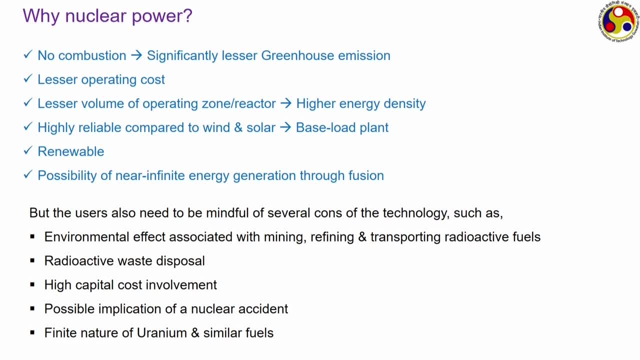 of electricity or energy that we get from a nuclear plant is independent of the surrounding condition and the demographic details and therefore they are excellent as base load power stations. They are not suffer too much by the fluctuations in the environment, The environmental conditions, and therefore they are easier to control, in a way also. 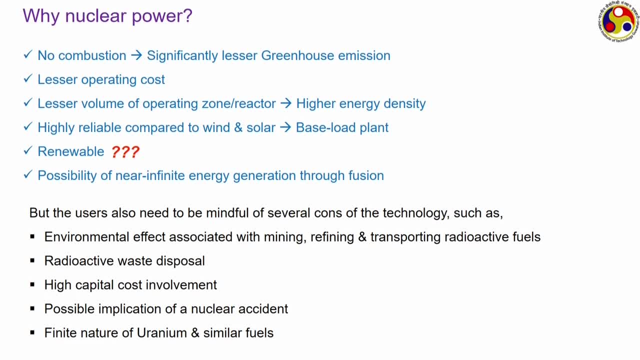 Next point may raise some eyebrows: renewable Now renewable, conventionally we attach these terms to solar, wind and biomass, but here I am using that on renewable with nuclear also. Well, I shall be coming back to this after a few lectures. but in certain situations, 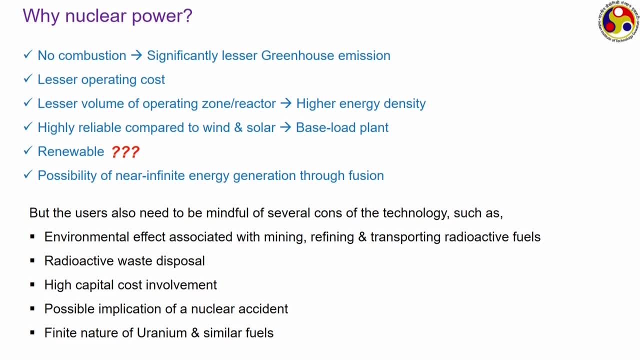 nuclear energy can also be termed as renewable, Then possibility of near infinite energy generation through fusion reaction. again, I shall be coming back to this later on, But just to put into the perspective, a projection shows that while the reserve of coal and other kind of fossil fuels may not last for more than 50-60 years. common nuclear fuels like uranium and thorium they also may not last more than 100 years. But if we use the fusion reaction, if you are able to master this technology, that can. 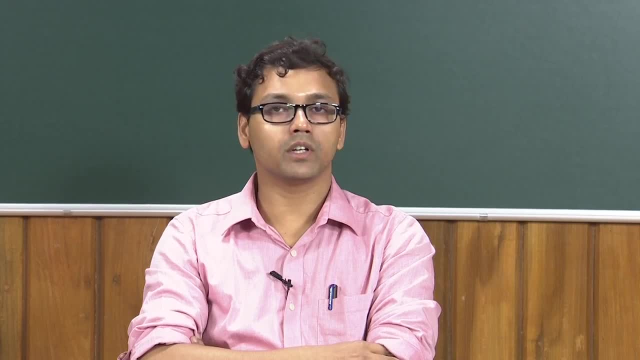 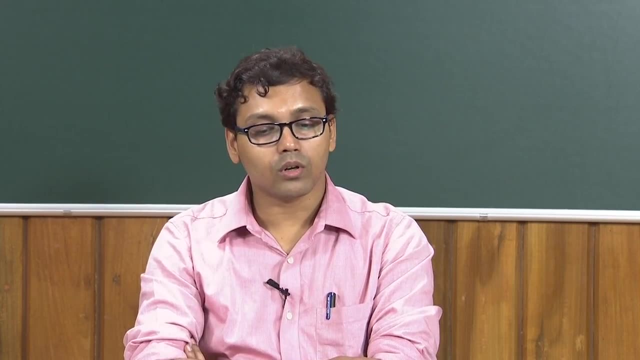 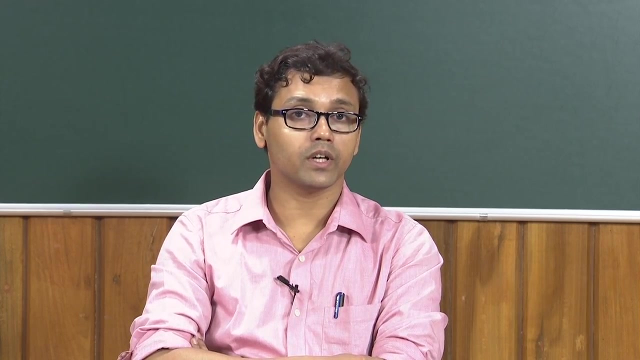 provide energy for about 300,0000 years. So how that, of course, we shall be discussing later on. But everything is not are we rosey about this nuclear power, because there are several factors that we need to be mindful of, like the environmental effect that everyone discusses about. 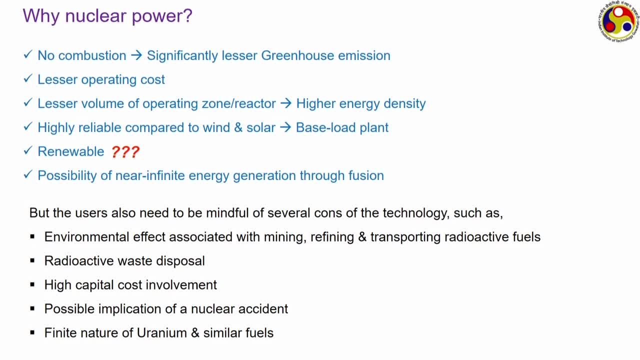 It is particularly with the handling of radioactive fuels, mining, refining and transportation of the same. There is possibility of radiation hazards in many places of the world. Module number 10, we shall be discussing about this: radioactivity and radioactive hazards and possible ways of getting us protected from that. 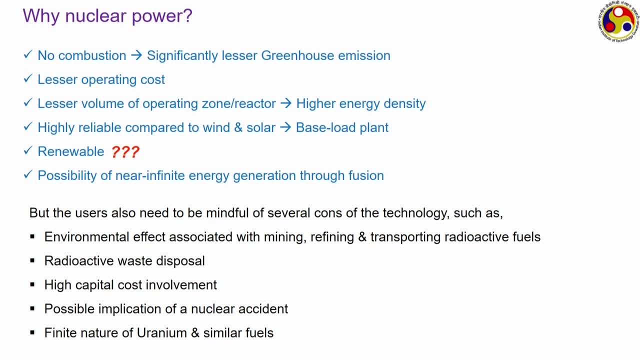 The radioactive waste disposal, the topic of the last module, and another very highly debated topic, The high capital cost involvement nuclear power plant, as that requires several layers of protection to protect us from the containment and other kind of radiation related issues. generally the capital cost involvement is much higher than fossil fuel based plants. The possible implication of nuclear accidents, while so far in the history there are only three incidents where accidents has happened in some nuclear power plant: The Three Mile Island in US in 1979, the Chernobyl incident, I think in 1985 or 86 in the former. 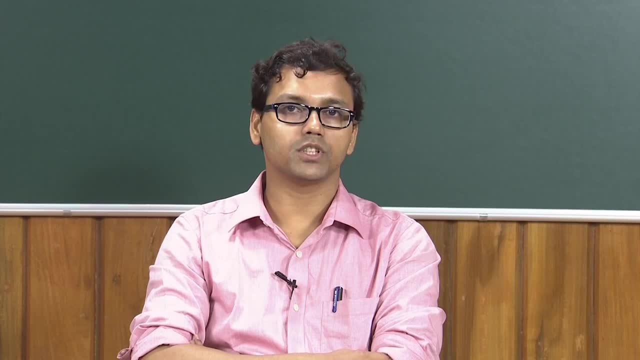 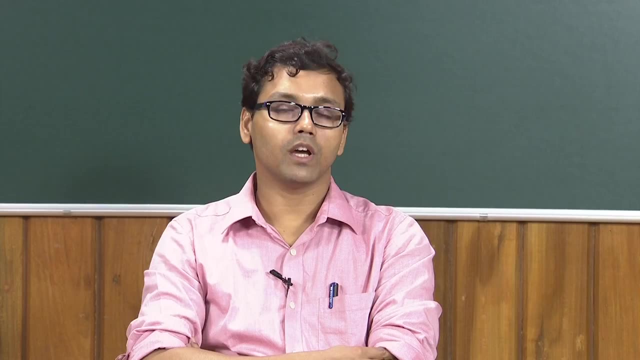 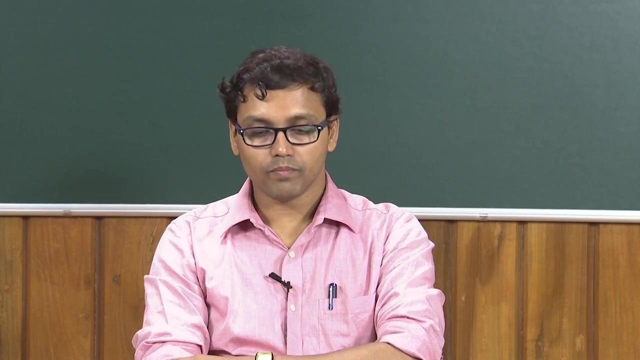 Soviet Union and the very recent one at Fukushima power stations. We shall be trying to discuss a bit about the details of each one, Each of them, and try to see how or they happened or what are the reasons behind each of those accidents and what are the factors. we need to be careful learning from them. 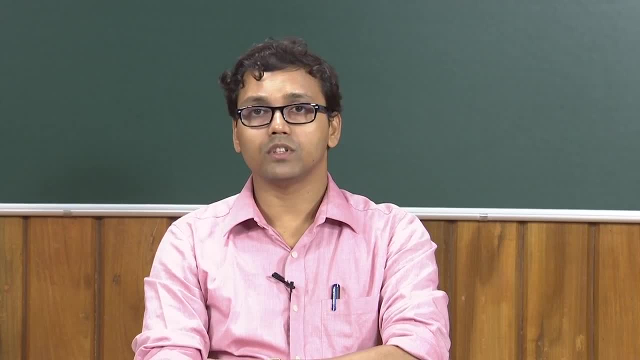 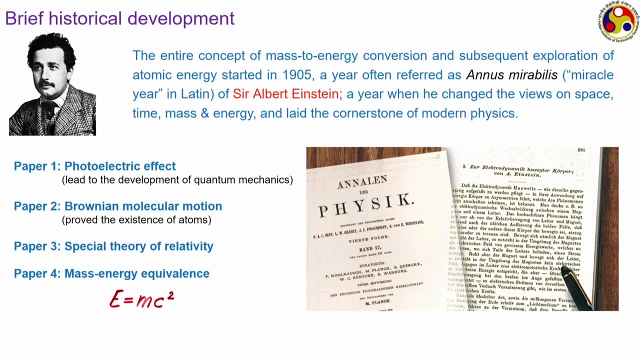 The finite nature of uranium and other fuels that is similar to the fossil fuels. that can also be a concern. So, with these factors in mind, let us now try to see a bit about historical development of the nuclear power generation, This being a fundamental portion of the history of the nuclear power generation. 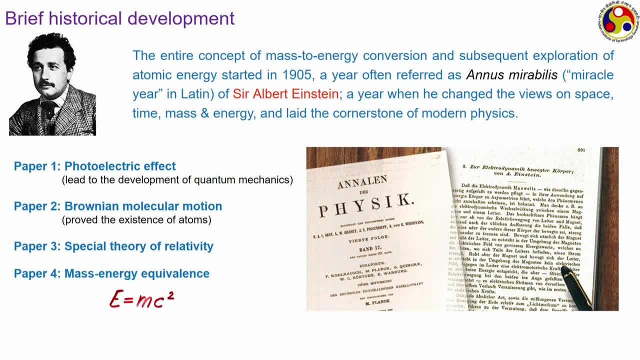 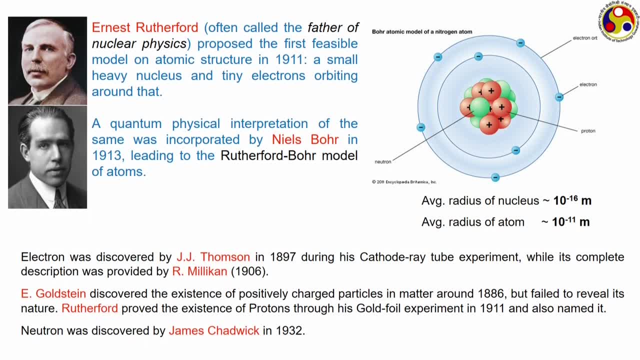 So let us now try to see a bit about historical development of the nuclear power generation. So Ernest Rutherford was the person which is often referred as the father of nuclear physics. He proposed the atomic structure. they give the first feasible model of atomic structure. 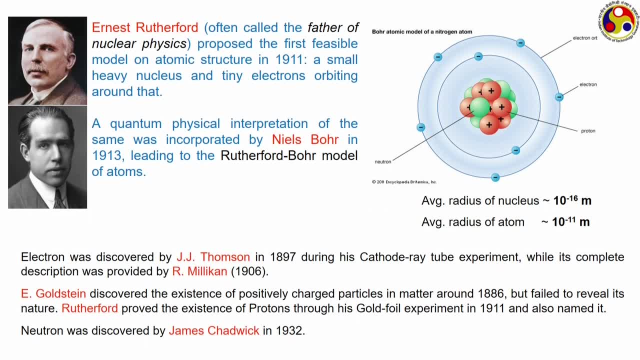 in 1911, which is quite similar to the solar structure that we have, or solar system where we have a heavier mass at the centre and all the electrons orbiting around that in elliptical or hemispherical, or I should not say hemispherical, semicircular kind of orbits. 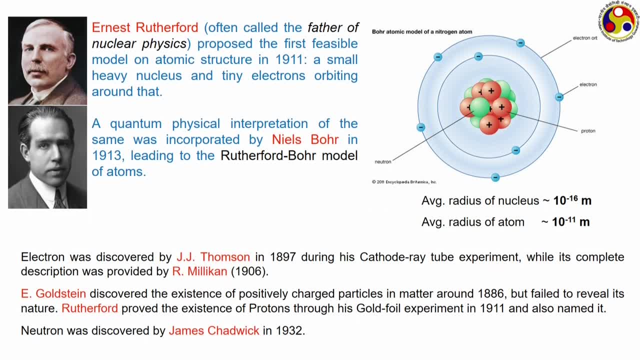 The heavier nucleus was identified to be positively charged and the mass of the nucleus was found to be much, much larger compared to the electrons. It was followed by the interpretation of Niels Bohr following the quantum physics, and therefore this model is often referred as the Rutherford Bohr model of atoms. 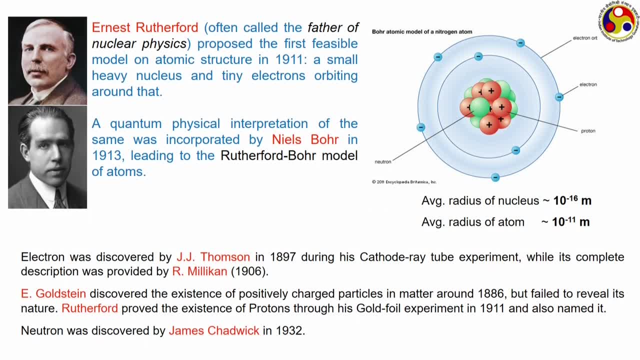 Their work established that inside the atoms there is a huge amount of empty space, because the average radius of nucleus was measured to be in the range of 0.5 to 0.5 nanometer, or in the range of 10 to the power minus 16 meter, whereas the average radius of atom 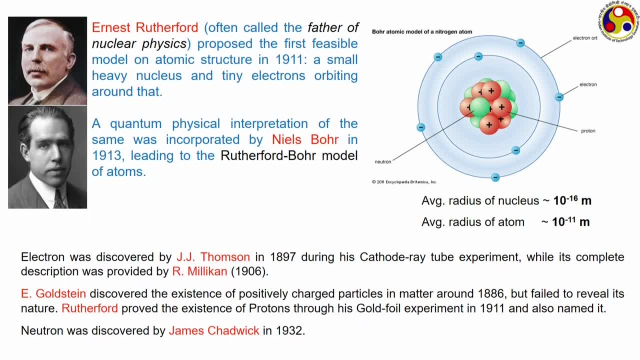 is of the order of 10 to the power minus 11 meter, and this huge amount of space inside was occupied only by very, very tiny electrons. This empty space is very, very important, which we shall be discussing later on. There are several subatomic particles which are present inside the nucleus, particularly 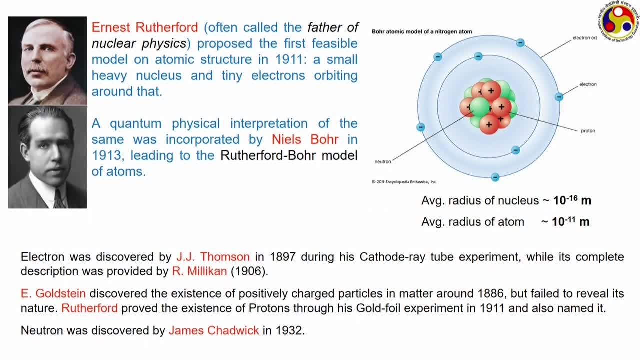 in the present age of gravitational wave, We should mention about positrons and neutrinos. So we will discuss about positrons, We will discuss about neutrinos, but here I am not not going to mention about those, because in this particular course we shall be restricting ourselves only to this three. 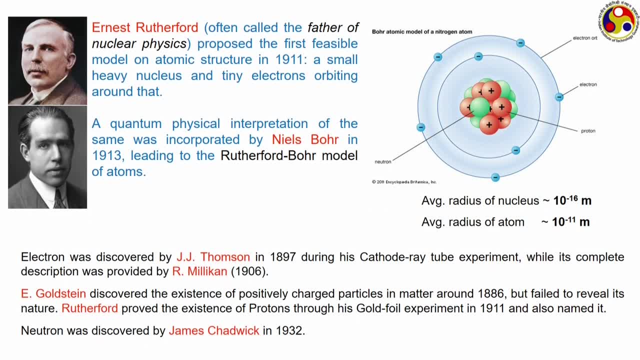 well known subatomic particles: proton, neutron and, of course, electron. Electron was discovered by J J Thomson in 1897 during his cathode ray experiments, and the complete description of electron, particularly the measurement or idea about its mass and energy, was given by R Millikan in around 1906. 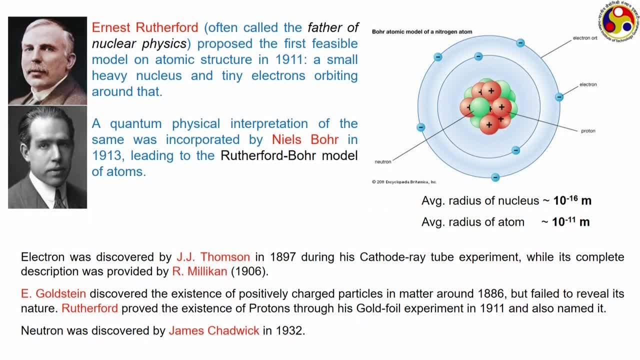 Goldstein was the researcher who discovered the existence of positively charged particle inside the matter. It was around 1886, but he failed to reveal the nature or completely. he was not able to completely describe the nature of this positively charged particle. Rather, he proved the existence of protons through his gold foil experiment in 1911. and 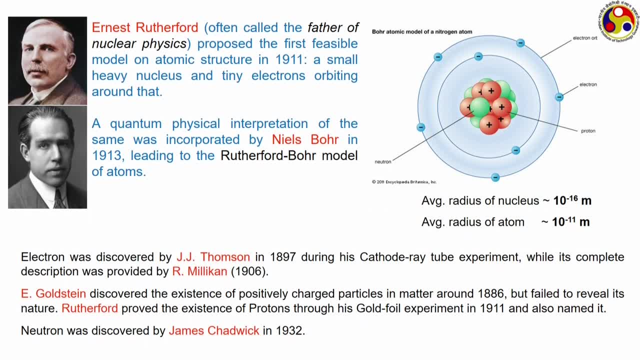 also, he gave the name proton, but it was also identified that nucleus does not constitute only proton, It is a body of protons. but there it is possible to have some other heavy subatomic particle which probably is neutral. and from the discovery of that neutral element was 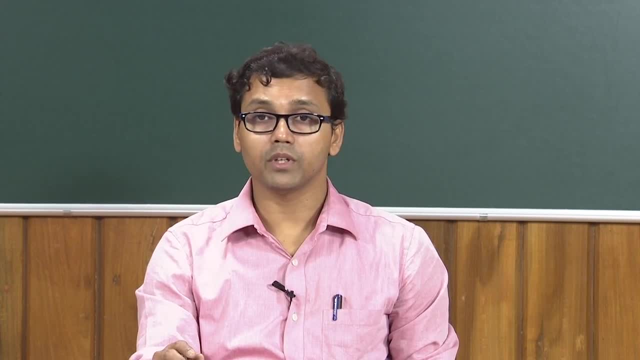 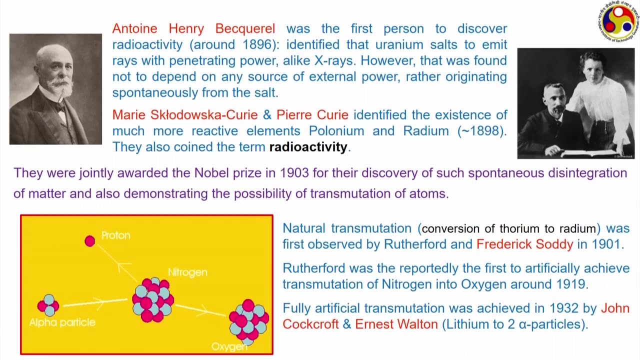 done by James Chadwick in 1932, and it was named neutron, and this particular discovery has far reaching implication on the development of nuclear physics. Henry Becker was the person who first discovered the concept of radioactivity around 1896, when he identified that uranium salt can emit rays with penetrating power which are quite similar. 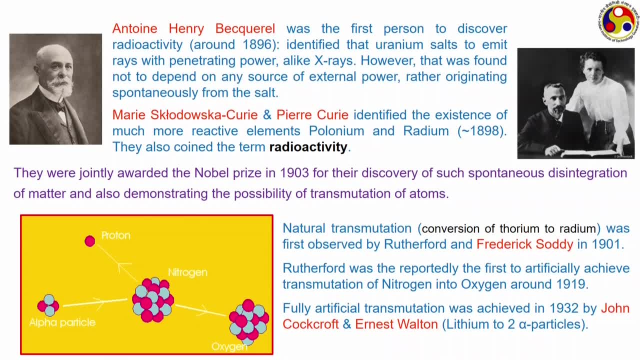 to X-rays, but they do not need any kind of external power to produce that. rather, that was found to be coming out more spontaneously from the salt. Simultaneous experiments are also done by the Cury family, that is, the Madame Cury and Pierre Cury. they identified the existence of much more reactive elements. 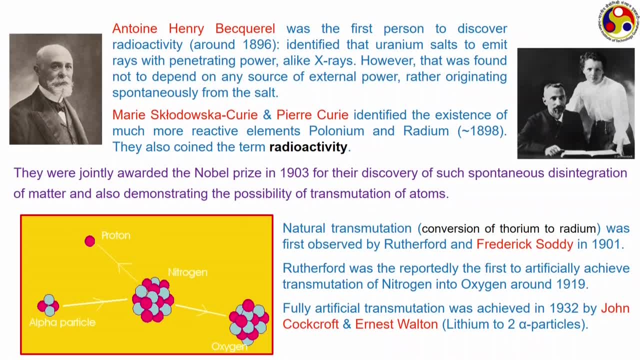 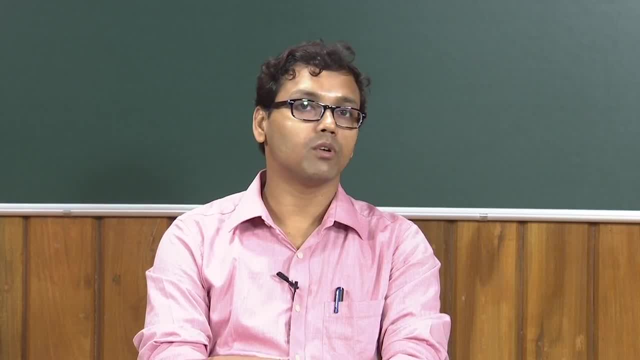 They were the persons who coined the term radioactive element, So they have also been selected as a way of using the term radioactive element. find the term radioactivity, and they also identified two radioactive elements which are found to be much more reactive compared to uranium, and they gave the name polonium. 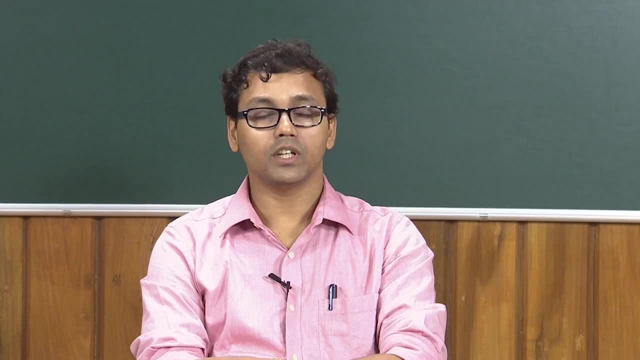 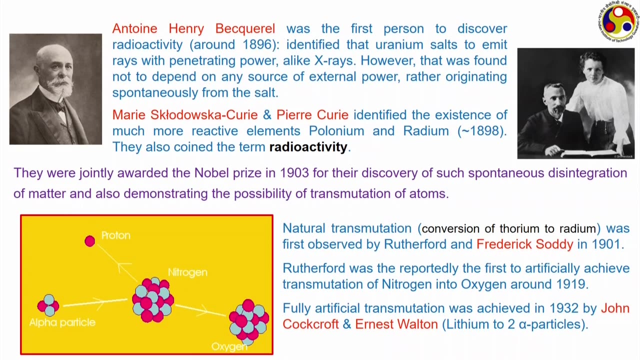 and radium. Radium was discovered around 1898. The name polonium actually refers to Poland, which was the birthplace of Madame Curie. Both Becquerel and Curie family together received the Nobel Prize in 1903 for the discovery of the radioactivity or spontaneous disintegration. 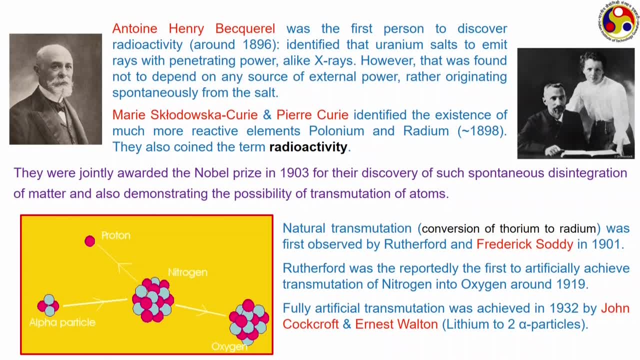 of matter. but this was only the natural phenomenon of spontaneous disintegration, Natural transmutation of atoms, that is, conversion of one atom to the other. that was first observed by Rutherford and Frederick Sodie in 1901.. Rutherford, repeatedly, was reportedly- Rutherford was the first person. 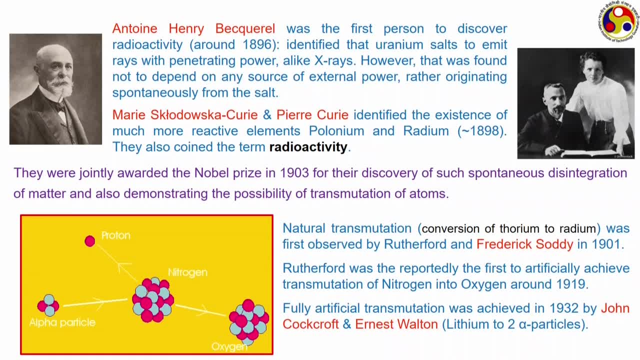 to achieve artificial transmutation of nitrogen to oxygen around 1919, but fully artificially. transmutation was achieved in 1932 by John Cockcroft and Ernest Walton, when they were able to convert lithium to two helium atoms, which led to several groups actively working on this topic of transmutation, that is, converting one atom to another and thereby releasing 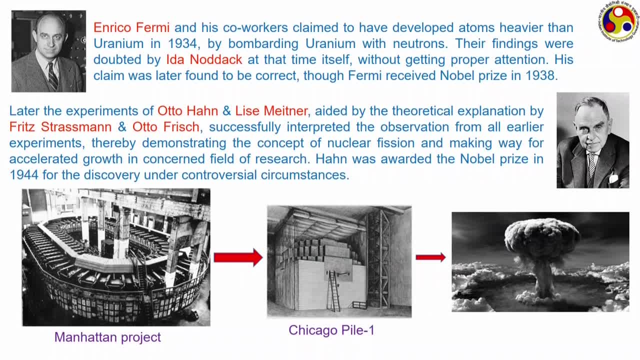 the energy stored in the atom. Enrico Fermi and their his co-workers were the group who first claimed to have developed atoms heavier than urea in 1934. Because, till that time, uranium was the atom known to, was identified as the atom with the. 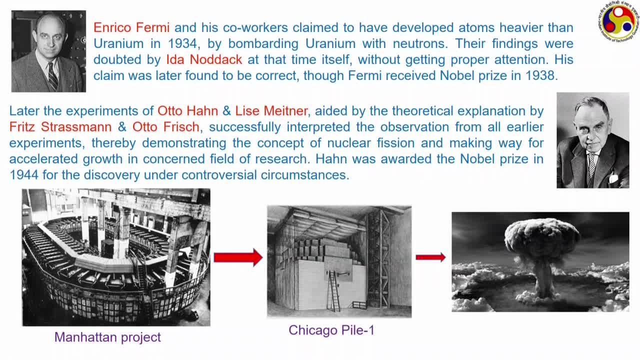 heavier mass or the highest amount of mass, but Fermi claimed that they have discovered atoms higher than this by bombarding uranium with neutrons. Their claim was: neutron has absorbed the uranium. or sorry, uranium has absorbed the neutron, thereby converting it to much heavier atom. 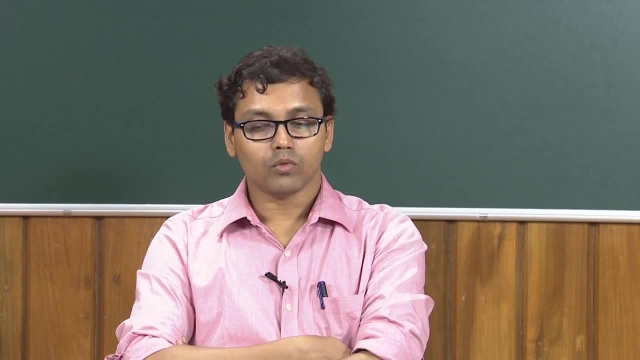 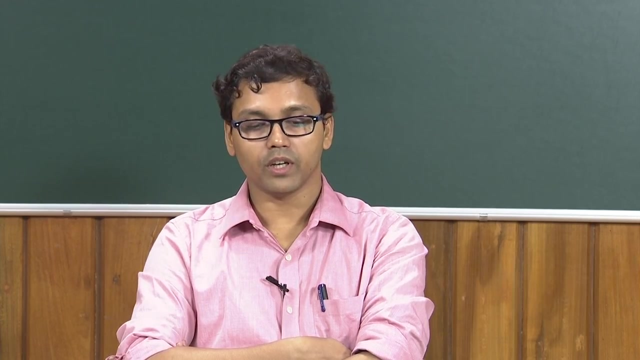 And developing a newer atom. but their claim was doubted by Idi and elegPEM at the same time itself, but that failed to attract proper attention. His claim led to the led to the nobel prize in 1938, but later on it was proved that Fermi's experiments was wrong, or rather 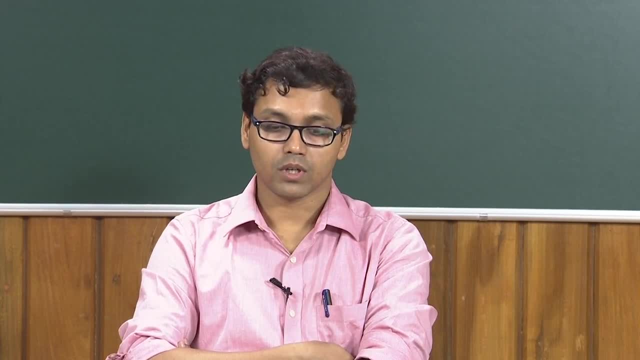 Fermi's interpretation of the experimental observation were wrong. The experience of Otto Hahn and Leis-Matzner added to the Freddy's simple topics and this made the Terra-Citimizee experiment much more meaningful In terms of the experiments. the experiments. 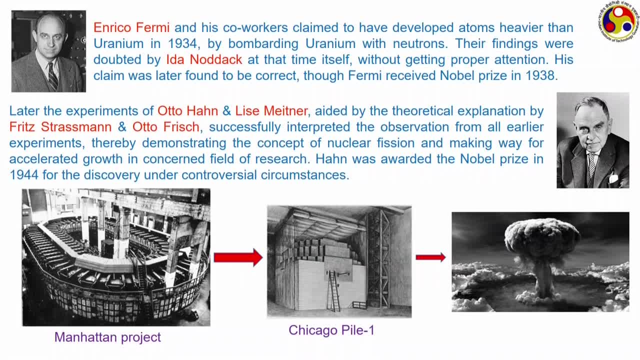 And they for contributed, or they continue to work on this particular field for several years, and they were the first group. aided by the theoretical explanation provided by Fritz Strassmann and Otto Fritz, They successfully interpreted the observations from all earlier experience, including that from Fermi and their co-workers, and were able to achieve a proper nuclear reaction under 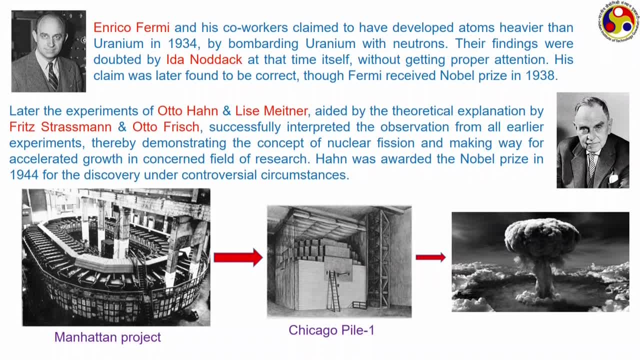 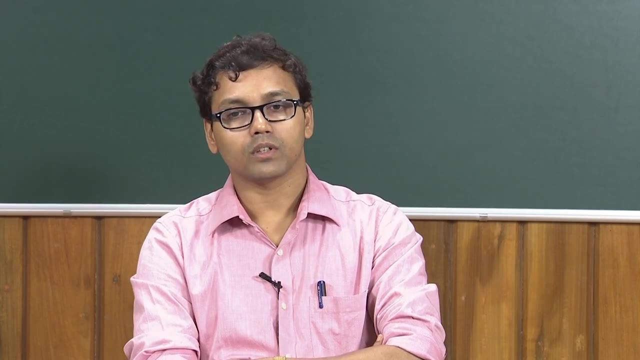 controlled condition and also liberate the energy that is stored in the atom. Their work led to the Nobel Prize of Otto Hahn in 1944, which was given under quite controversial circumstances, because this Nobel Prize was awarded or announced in the later part of 1945, post the Second World War, where the atom bomb at Hiroshima and Nagasaki was already. 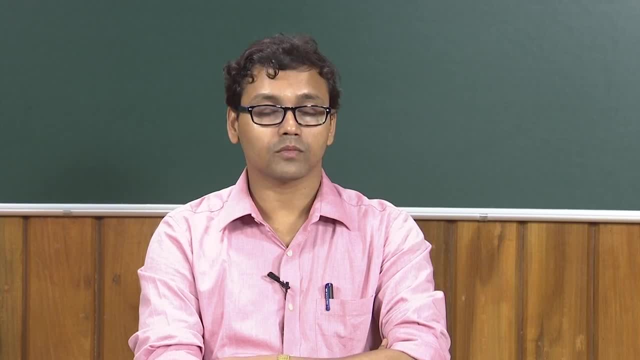 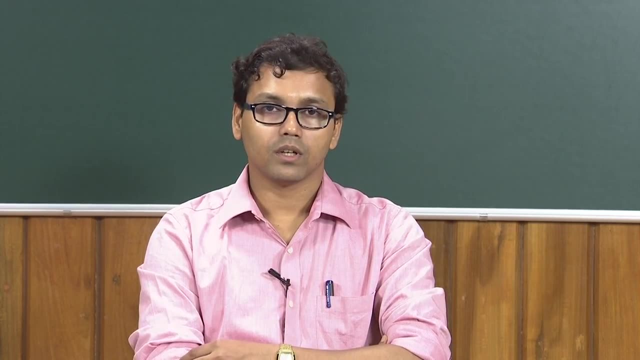 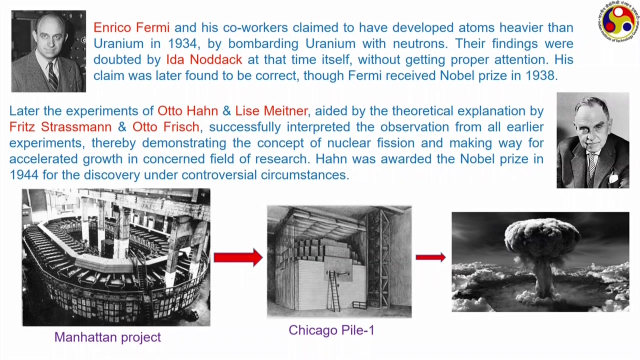 history And Otto Hahn was already a member of the Nobel Prize. He was also under the locker, or I should say he was in jail, and but it is also quite unfair to give the Nobel Prize only to the Otto Hahn, because Mitner and Strassmann contributed. 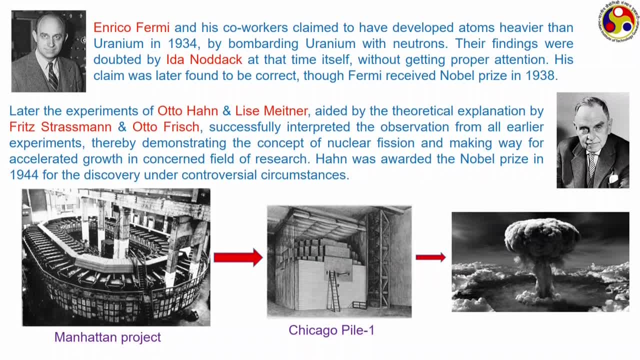 equally to the experiment, but still- Hahn was the person who received the Nobel Prize for this- and the result of their interpretation led to the Manhattan Project In Chicago, Pile 1, the first ever nuclear reactor developed by mankind, and then the unmentionable at the Hiroshima in 1945. 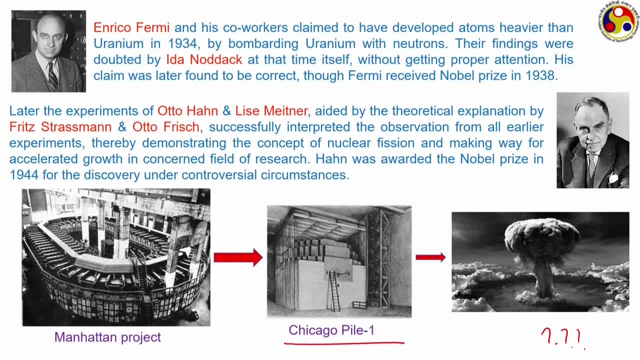 Thankfully, scientists did not stop there. rather, they continued working on this and did not restrict nuclear energy only to the weapons, rather started thinking about using this huge amount of energy source for the benefits of the mankind. And they did not restrict nuclear energy only to the weapons, rather started thinking about 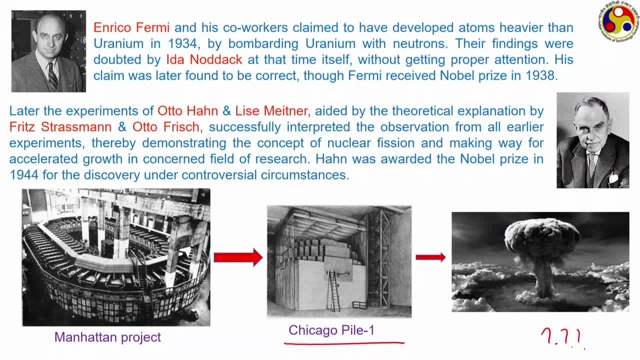 using this huge amount of energy source for the benefits of the mankind. And they did not restrict nuclear energy only to the weapons, rather started thinking about using this huge amount of energy source for the benefits of the mankind. And they did not restrict nuclear energy only to the weapons, rather started thinking about. 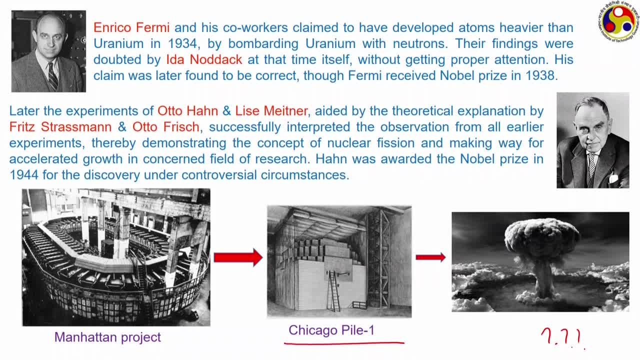 using this huge amount of energy source for the benefits of the mankind. And they did not restrict nuclear energy only to the weapons, rather started thinking about using this huge amount of energy source for the benefits of the mankind. And they did not restrict nuclear energy only to the weapons, rather started thinking about. 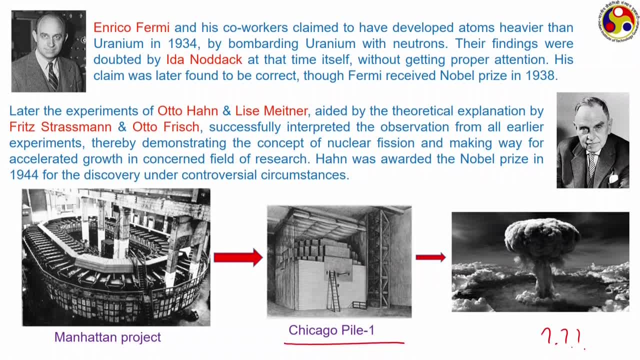 using this huge amount of energy source for the benefits of the mankind. And they did not restrict nuclear energy only to the weapons, rather started thinking about using this huge amount of energy source for the benefits of the mankind. And they did not restrict nuclear energy only to the weapons, rather started thinking about. 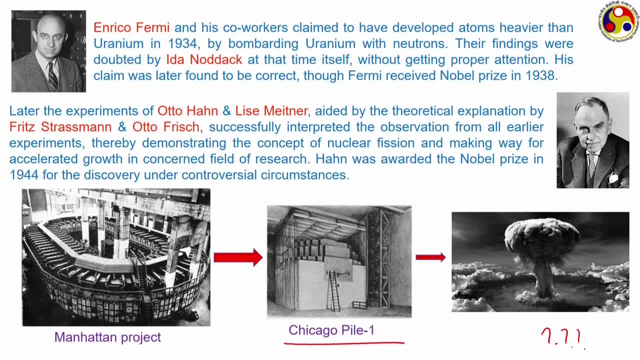 using this huge amount of energy source for the benefits of the mankind. And they did not restrict nuclear energy only to the weapons, rather started thinking about using this huge amount of energy source for the benefits of the mankind. And they did not restrict nuclear energy only to the weapons, rather started thinking about. 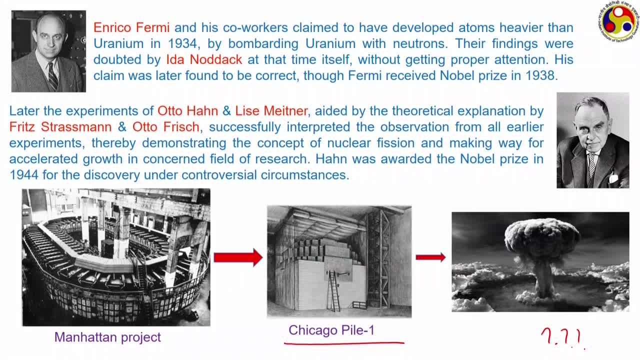 using this huge amount of energy source for the benefits of the mankind. And they did not restrict nuclear energy only to the weapons, rather started thinking about using this huge amount of energy source for the benefits of the mankind. And they did not restrict nuclear energy only to the weapons, rather started thinking about. 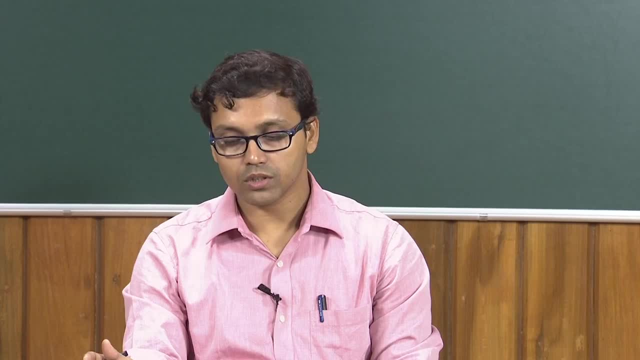 using this huge amount of energy source for the benefits of the mankind. And they did not restrict nuclear energy only to the weapons, rather started thinking about using this huge amount of energy source for the benefits of the mankind. And they did not restrict nuclear energy only to the weapons, rather started thinking about. 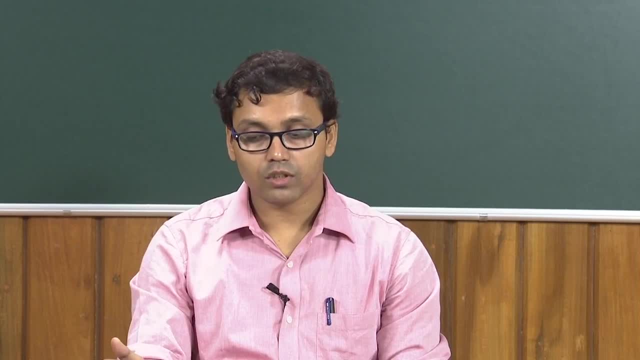 using this huge amount of energy source for the benefits of the mankind. And they did not restrict nuclear energy only to the weapons, rather started thinking about using this huge amount of energy source for the benefits of the mankind. And they did not restrict nuclear energy only to the weapons, rather started thinking about. 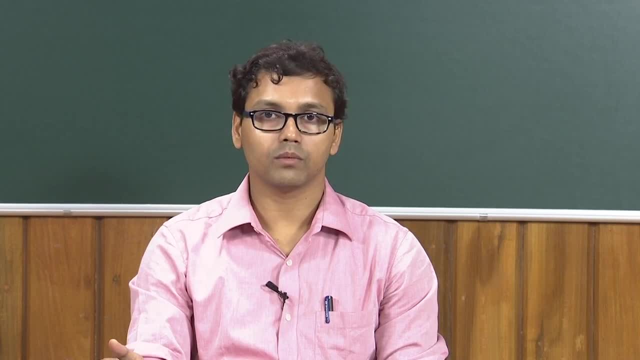 using this huge amount of energy source for the benefits of the mankind. And they did not restrict nuclear energy only to the weapons, rather started thinking about using this huge amount of energy source for the benefits of the mankind. And they did not restrict nuclear energy only to the weapons, rather started thinking about. 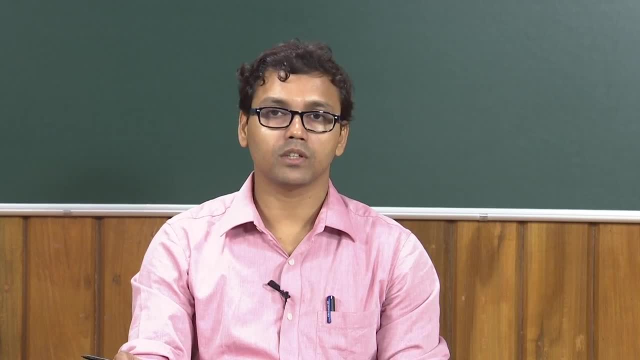 using this huge amount of energy source for the benefits of the mankind. And they did not restrict nuclear energy only to the weapons, rather started thinking about using this huge amount of energy source for the benefits of the mankind. And they did not restrict nuclear energy only to the weapons, rather started thinking about. 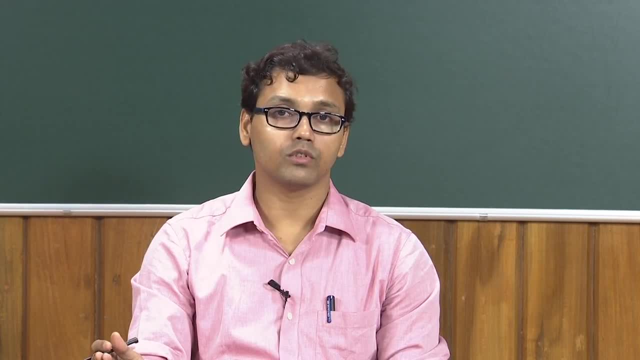 using this huge amount of energy source for the benefits of the mankind. And they did not restrict nuclear energy only to the weapons, rather started thinking about using this huge amount of energy source for the benefits of the mankind. And they did not restrict nuclear energy only to the weapons, rather started thinking about. 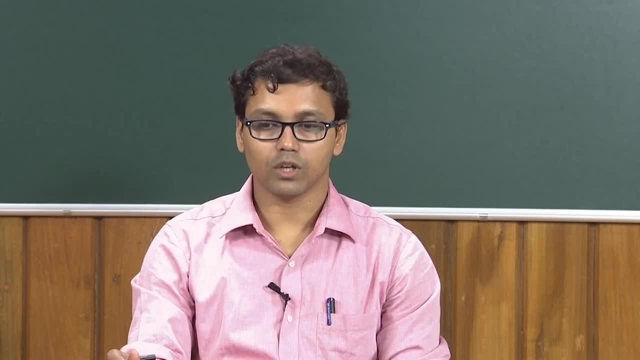 using this huge amount of energy source for the benefits of the mankind. And they did not restrict nuclear energy only to the weapons, rather started thinking about using this huge amount of energy source for the benefits of the mankind. And they did not restrict nuclear energy only to the weapons, rather started thinking about. 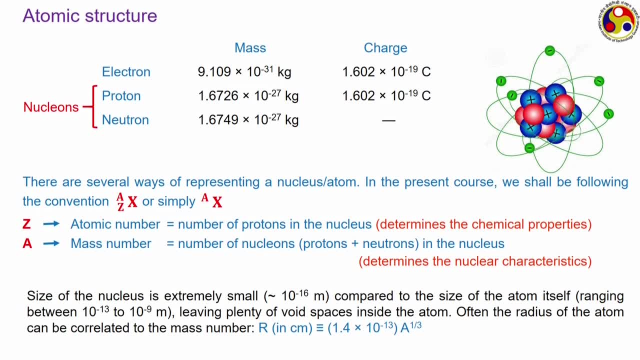 using this huge amount of energy source for the benefits of the mankind. And they did not restrict nuclear energy only to the weapons, rather started thinking about using this huge amount of energy source for the benefits of the mankind. And they did not restrict nuclear energy only to the weapons, rather started thinking about. 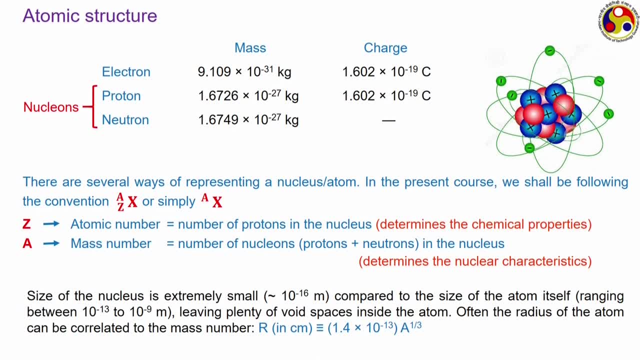 using this huge amount of energy source for the benefits of the mankind. And they did not restrict nuclear energy only to the weapons, rather started thinking about using this huge amount of energy source for the benefits of the mankind. And they did not restrict nuclear energy only to the weapons, rather started thinking about. 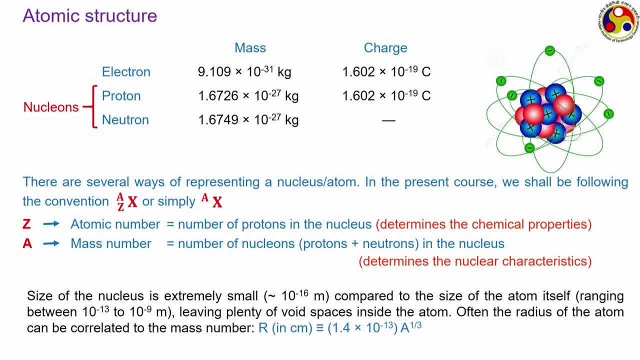 using this huge amount of energy source for the benefits of the mankind. And they did not restrict nuclear energy only to the weapons, rather started thinking about using this huge amount of energy source for the benefits of the mankind. And they did not restrict nuclear energy only to the weapons, rather started thinking about. 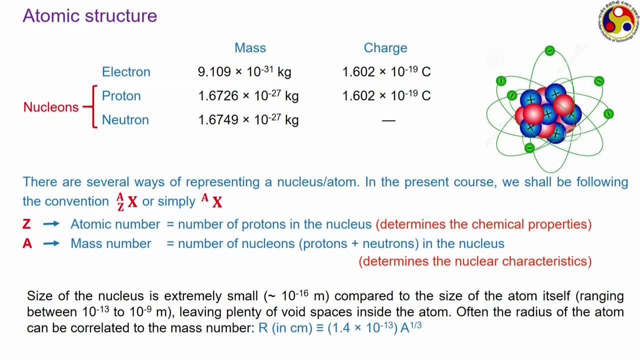 using this huge amount of energy source for the benefits of the mankind. And they did not restrict nuclear energy only to the weapons, rather started thinking about using this huge amount of energy source for the benefits of the mankind. And they did not restrict nuclear energy only to the weapons, rather started thinking about. 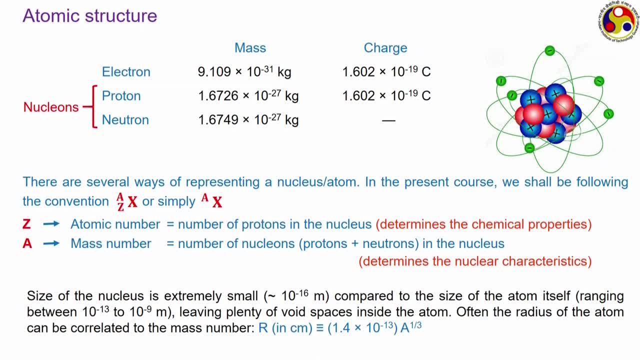 using this huge amount of energy source for the benefits of the mankind. And they did not restrict nuclear energy only to the weapons, rather started thinking about using this huge amount of energy source for the benefits of the mankind. And they did not restrict nuclear energy only to the weapons, rather started thinking about. 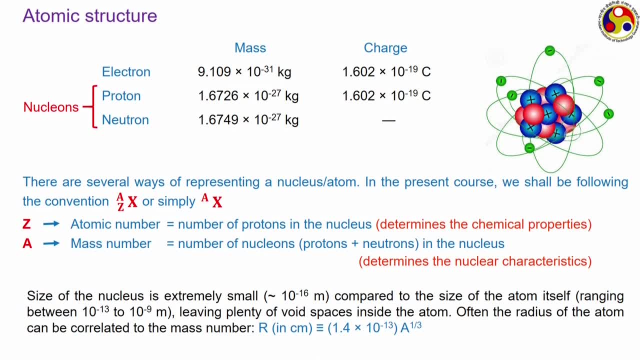 using this huge amount of energy source for the benefits of the mankind And they did not restrict nuclear energy source for the benefits of the mankind. The electrons are extremely small in terms of their mass. as you can see here, their mass is of the order of ten to the minus 31 kgs, whereas the nucleus comprises of proton and 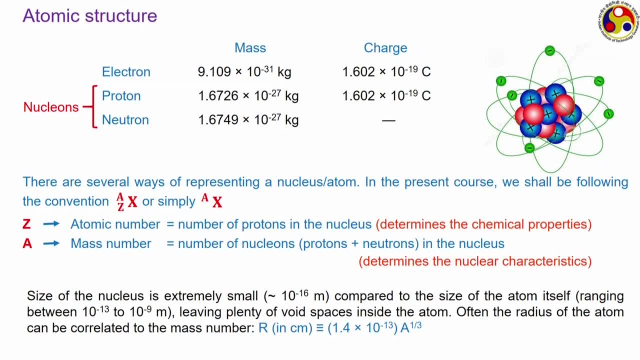 neutrons, who are having nearly similar mass, and it is of the order of 10 to the minus 27 kg, which is 10 to the power, 4 kg higher than electrons. And therefore, whenever we shall be doing any calculation from now on, or see using the 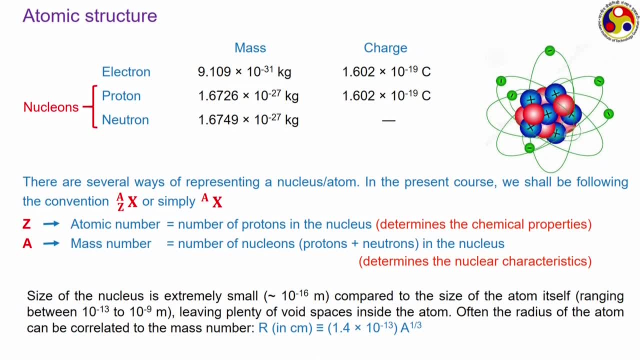 mass of proton and neutron. mass of the electron will invariably be neglected. Neutron is positively charged, whereas proton is having equal amount of charge as the electron, which is 1.602 into 10 to the power minus 19 coulomb. but the charge of proton and electron are of opposite sense. 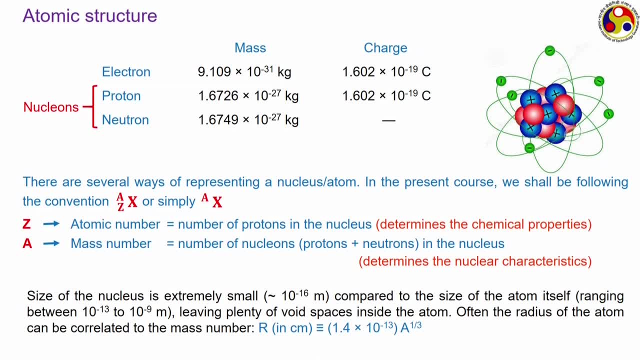 And therefore they are given opposite signs. conventionally, proton is called positively charged, whereas electron is called negatively charged. And proton and neutron, as both of them comprise the nucleus, they together are often called nucleons. Now there are several conventions by which we can represent a nucleus or an atom. In the present course. 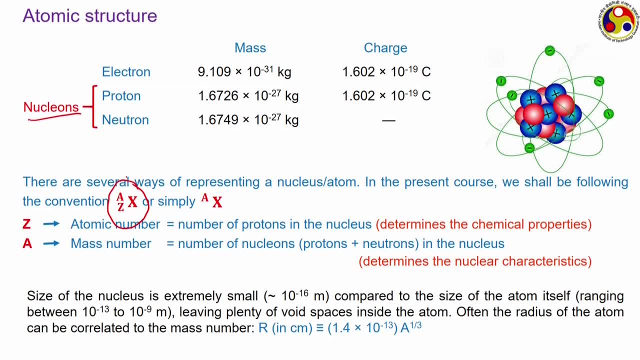 we shall be following this particular concept: A z x or A x z. Here z is the atomic number, which is equal to the number of protons present in the nucleus. So atomic number is the number of protons present in the nucleus, which, of course, is equal to the number of protons. 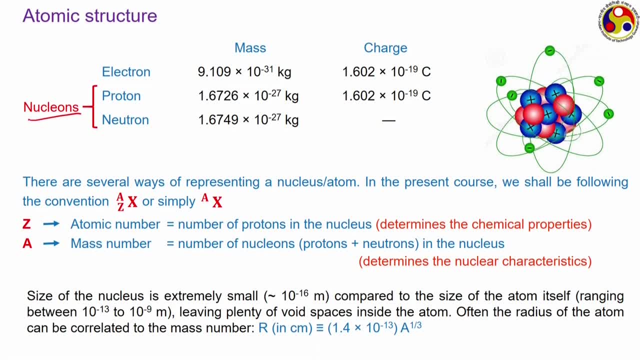 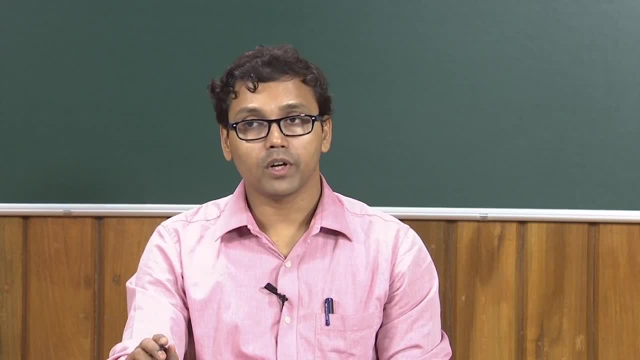 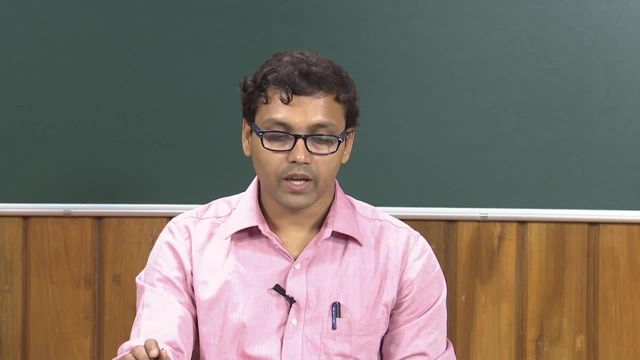 and the number of electrons rotating in the orbits to keep an atom electrically neutral. And it is the proton which generally determines the chemical properties of any particular nucleus And therefore atomic number is associated with the chemical properties. A, on the other hand, is the mass number, which is the total number of nucleons, that is, number of protons. 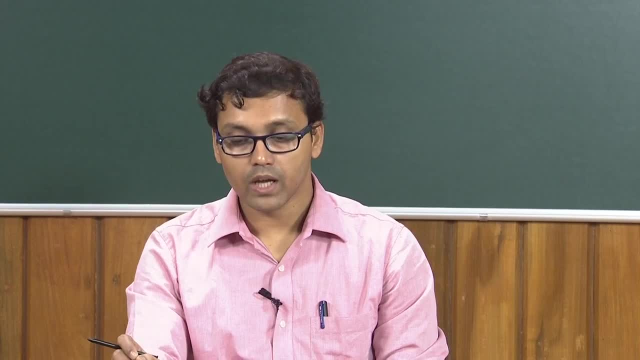 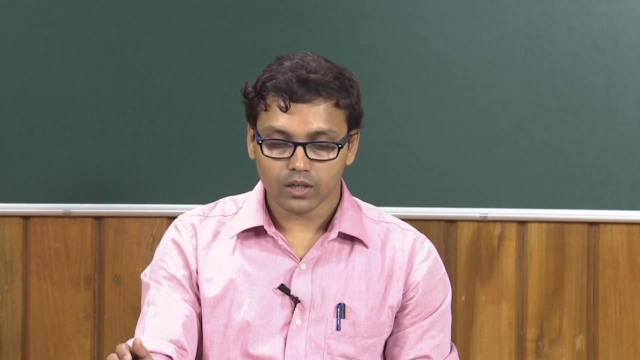 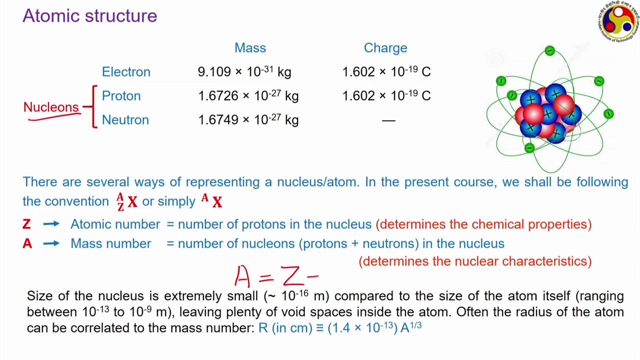 plus neutrons present together inside the nucleus. It determines the nuclear characteristics which we shall discuss later. We shall be repeatedly discussing in this course So the atomic number. we can write that the mass number is related to the atomic number plus the number of neutrons, which is 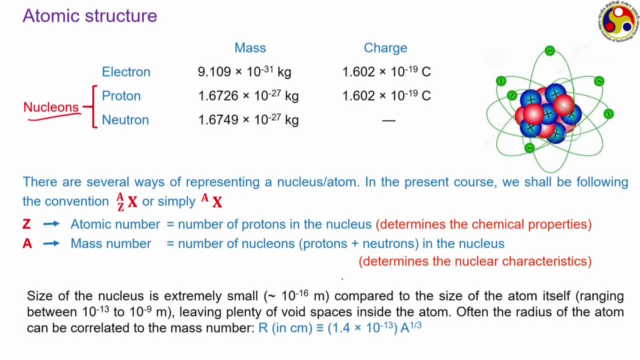 often represented by the symbol n. Now, the size of the nucleus is extremely small. as I have mentioned, It is of the order of 10 to the power minus 16 meter, whereas the size of the atom ranges from 10 to the power minus 19, to 10 to the power minus 13 meter, leaving 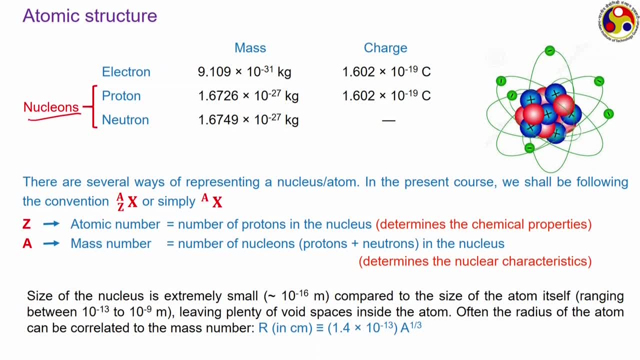 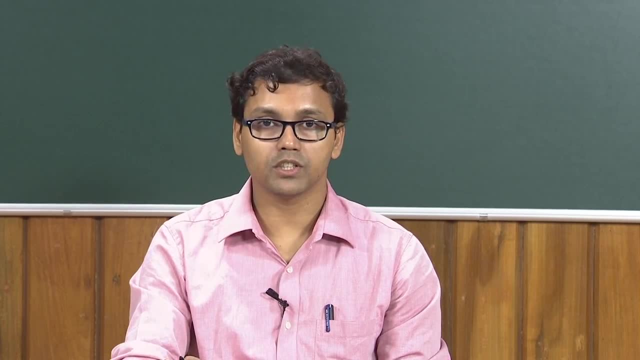 plenty of void space inside the atom. Quite often the radius of an atom is correlated to the mass number by a very much empirical relation like this: 1.4 into n to the power minus 13 into a to the power one third. But this is an empirical nature, relation of empirical nature and the radius that we get from atom. 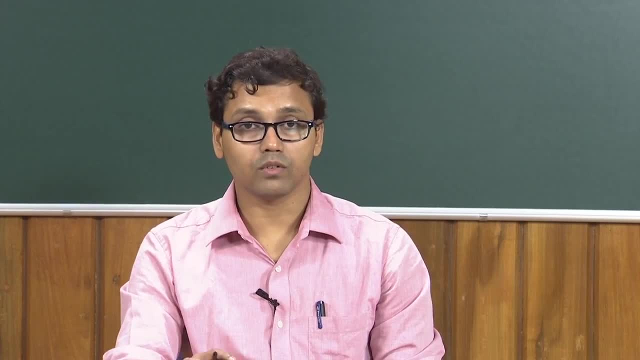 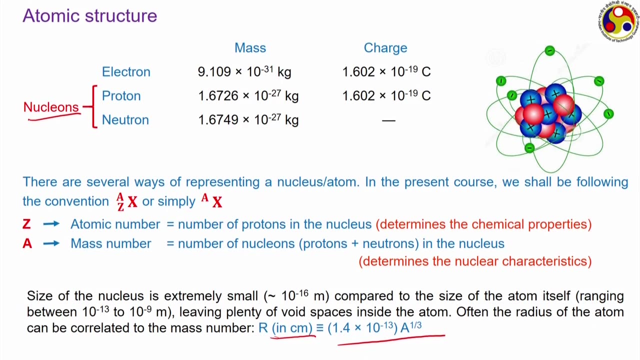 that is in centimeter. So please be careful about the unit of this radius. Now, both the isotropic various mass are calculated by the load weight property of the atomic number, which should be a relatively small unit of mass, which should be deine atoms. 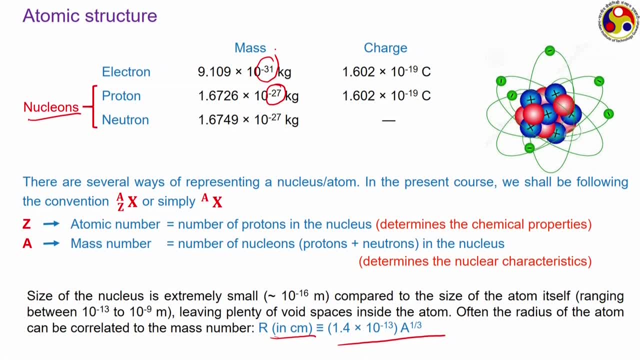 So. so I shall discuss the mass number here also. In particular, as we have seen the previous slide, here we are talking about extremely small mass, of the order of 10 to the power minus 27 kg, or of 10 to the power minus 31. 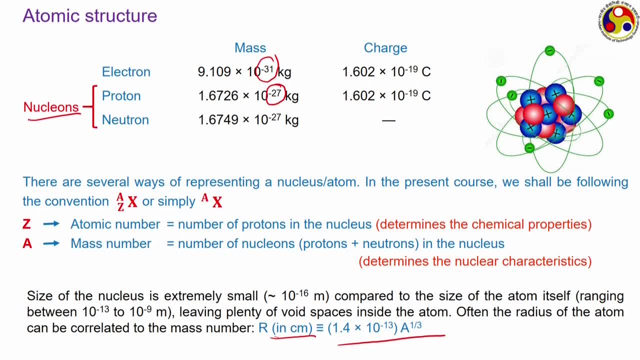 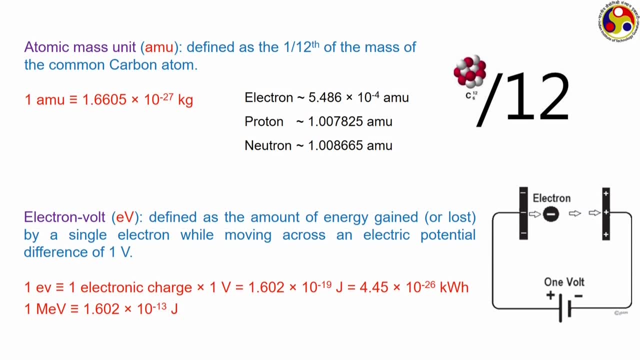 kgs, which are quite odd to discuss about using from the point of view of our day to day life, And therefore a new unit of mass is required to be proposed, and that unit is called atomic mass unit or a mu. are a mu, which is defined as 5.6 folds, which does give us a radius 1 vez to up to 125 cubic meter square. Now we will go through the istogeal personality of this, his model, which we will use Tool. this is specifications foroku спасибо. the euro By which the Tonal 120 sangat mesha by the. 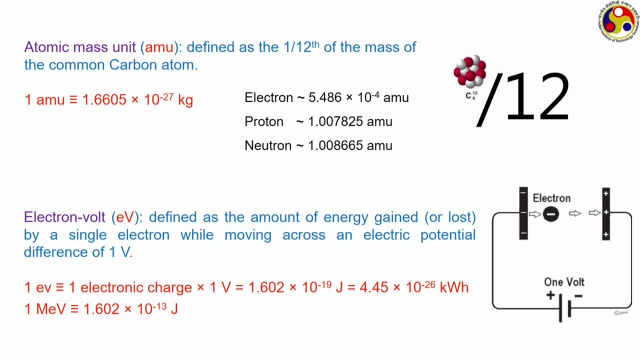 as one twelfth of the mass of the common carbon atom. Proper measurement says that one A mu is equal to 1.6605 into 10, to the power minus 27 kgs, which subsequently gives the mass of electron, proton and neutron as like this. So from now onwards we shall be using A mu. 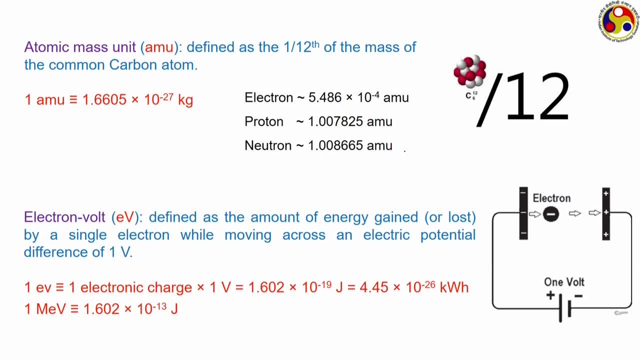 as the mass for energy. While A mu is a commonly used unit for this, but in some books you will also find a small u is used to define the mass of this atomic, subatomic elements. We shall also be proposing an unit for energy, which is electron volt. It is defined as the 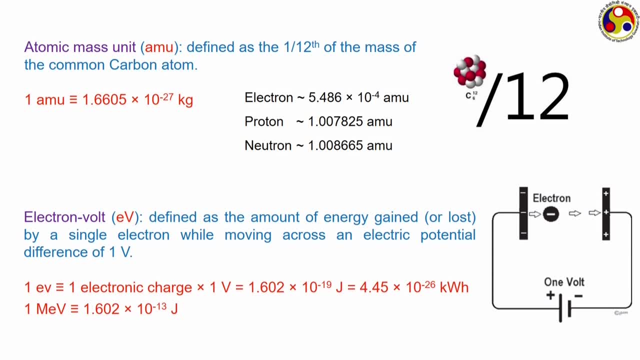 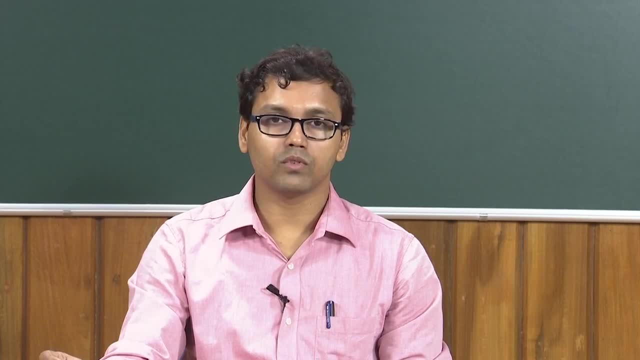 amount of energy gained or lost by a single electron as it passes through an electrical potential barrier of 1 volt. One electron passing through a potential barrier of 1 volt, then the amount of energy gained by the electron or amount of energy reduced by the electron. 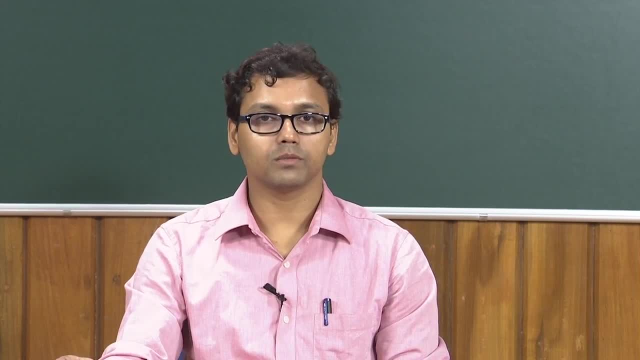 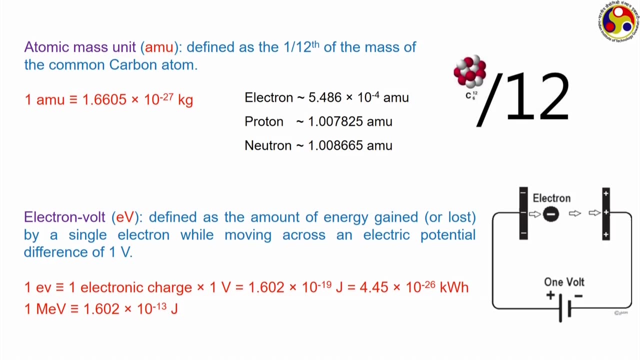 required to make it move is called one electron volt. So corresponding amount of energy will be one electronic charge multiplied by 1 volt, giving 1.602 into 10 to the power minus 19 joule. And electron volt generally being a small unit, one on MeV is mega electron volt, which is 1.602 into 10 to the power minus. 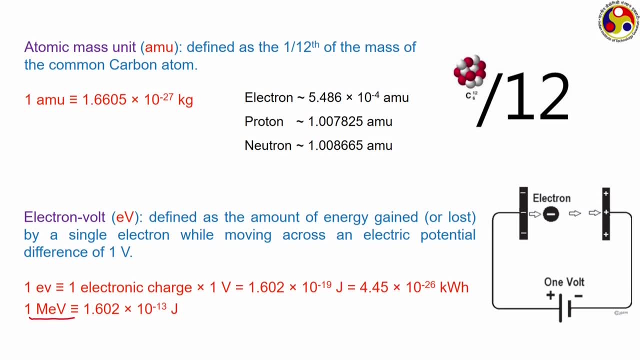 13 joule, We have to repeatedly make use of this particular one. So from now onwards we shall be using A mu as a unit for energy. So this is the unit for mass and MeV as the unit for energy, unless otherwise required. 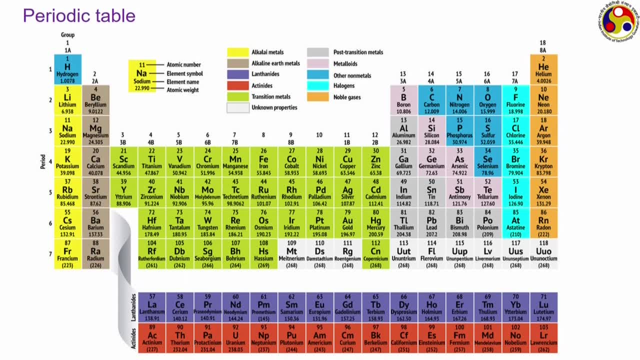 This is a structure of a modern periodic table where means this particular one shows elements up to an atomic number of 118, but truly speaking, up to atomic number of 92, which is uranium. Beyond that, basically all of them are artificial that is produced in the laboratory via some kind of nuclear experiments or nuclear reactions. but till 92 all the elements are naturally available. Hydrogen is the smallest one, or the first one in the series, which is having an atomic number of 1 and also a mass number of 1, because its nucleus contains only a single. 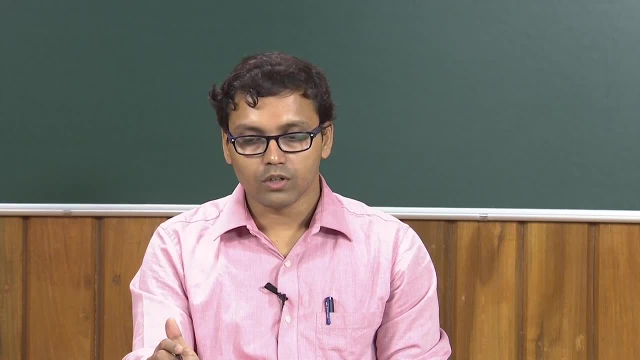 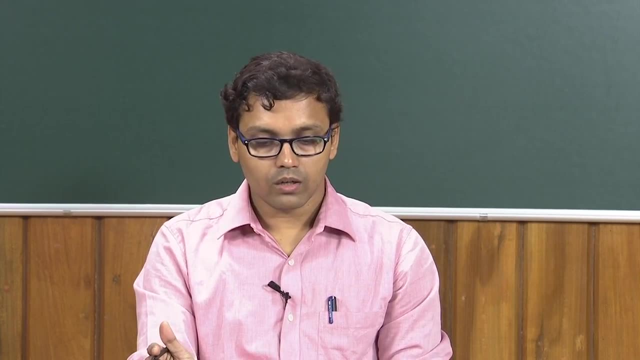 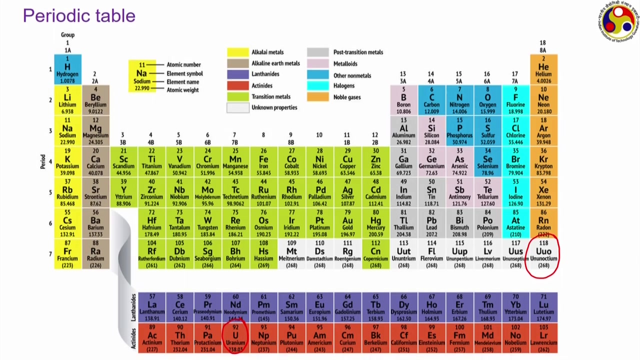 proton and no neutron. The next one is helium, which contains two protons and two neutrons, and that goes on this way. So, as we are discussing about radioactivity and nuclear reaction in this course, our interest will mostly be starting from the elements after lead. 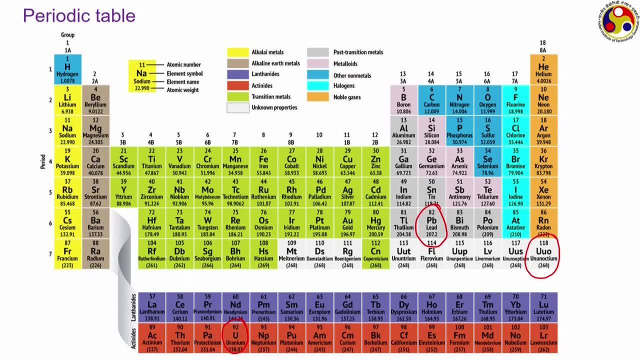 Lead is more or less nuclear. I should say it is neutral from nuclear experiments point of view. but all those elements after that, like this polonium and radon and radium, uranium, thorium, plutonium, they all are highly radioactive. 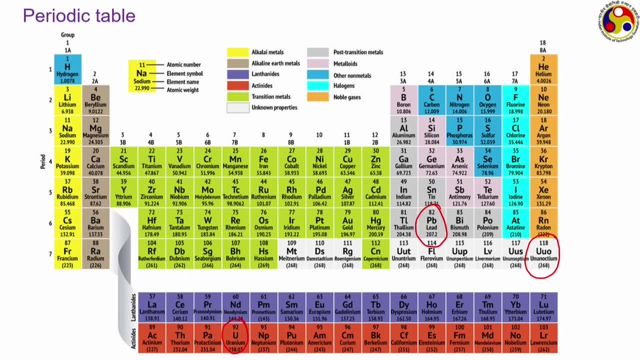 Of course their radioactivity level varies, but generally our discussion, at least in the first part of this course, will mostly be around this: materials after lead. But that is means. here of course we are showing the means. you can see here each of the symbols. 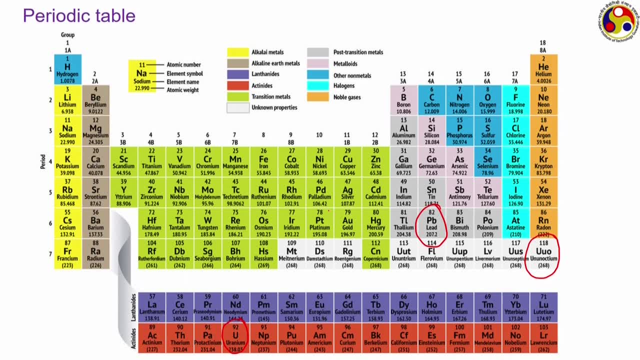 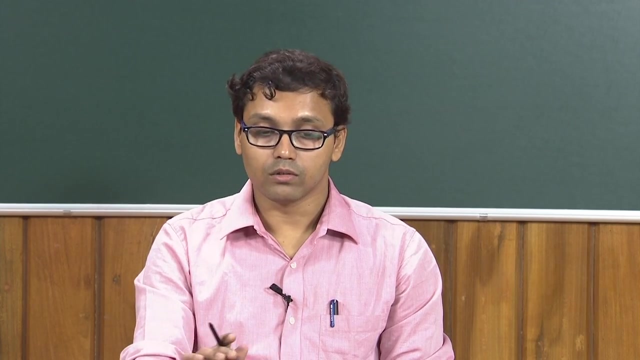 are followed by one number, like if we take, say, oxygen. here below the symbol we are presenting the mass number of common oxygen nucleus in terms of AMU, which is 15.999.. But this is only the common nucleus, but any atom can have multiple nucleus, which we call. 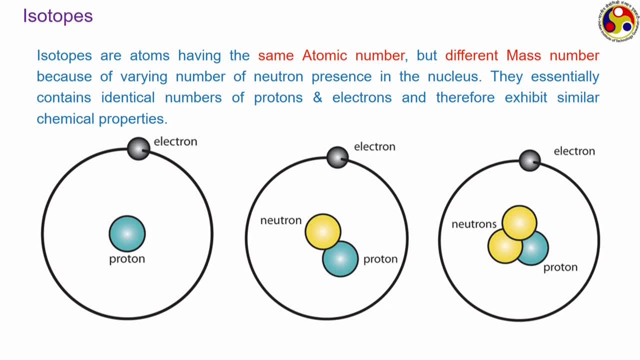 as isotopes, And isotopes are atoms which have the same atomic properties, Different number, but may have different mass number. that is, they have the same number of proton in the nucleus but may have varying number of neutrons. And, as we have already seen that protons are related to the chemical nature, 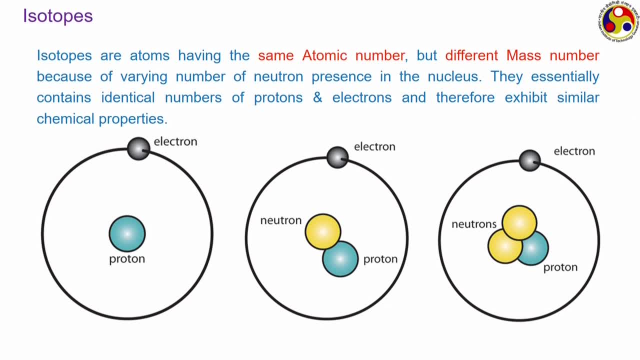 So their chemical properties will remain more or less the same, but the number of neutrons or number of nucleons that decides the nuclear nature, And therefore different isotopes of the same element may have different nuclear nature, while they are expected to have more or less the same chemical nature. 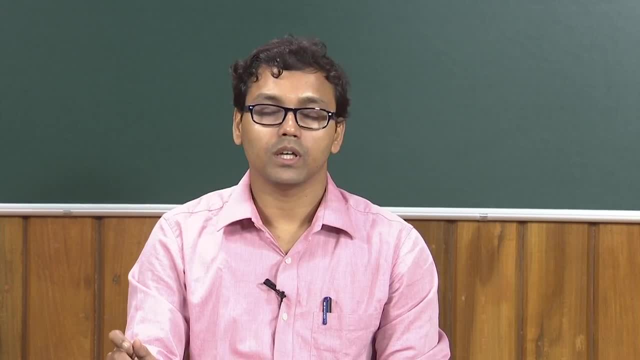 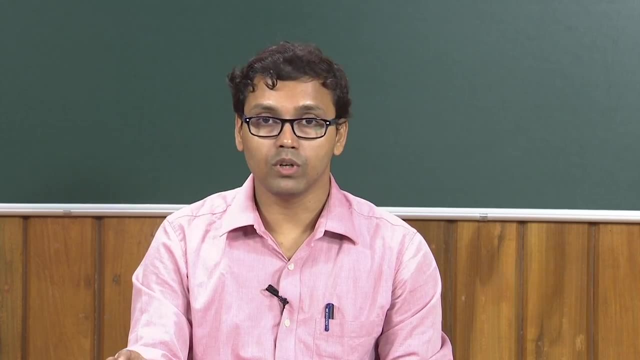 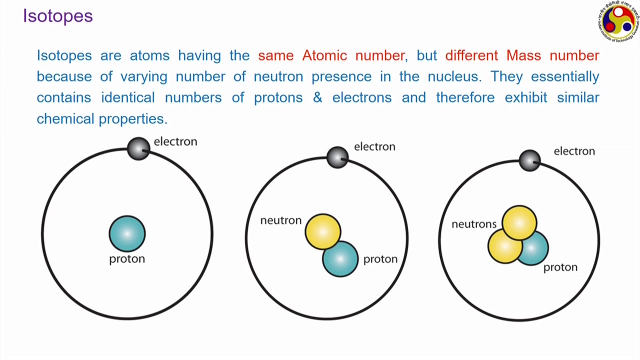 So, in a nutshell, by varying the number of neutrons in the nucleus, we can produce different isotopes of the same element and can vary their nuclear properties, Like here you can see three different isotopes of hydrogen: The first one, which is a common one, which has only a single proton and therefore one. 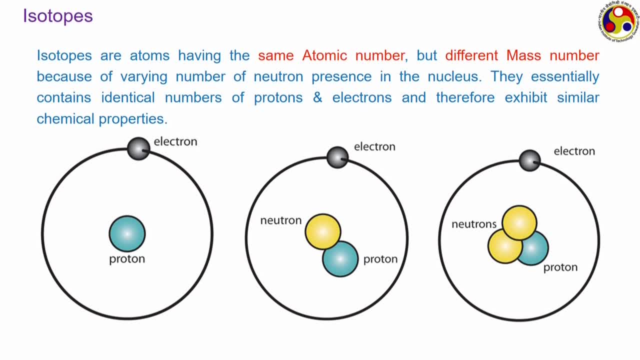 electron orbiting around that. no neutron in a nucleus, But in the second one, which is called deuterium, it has one neutron and one proton. So the atomic number is equal to the number of neutrons. So in a nutshell, by varying the number of neutrons in the nucleus we can produce different. 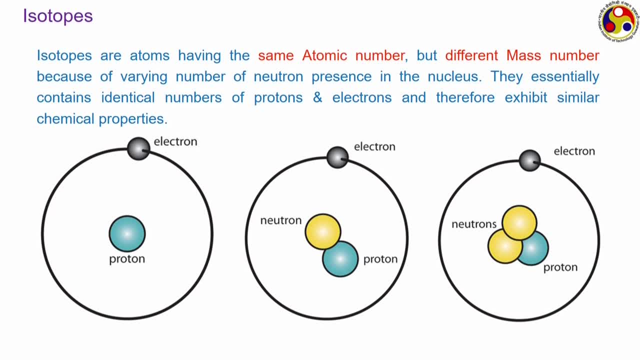 isotopes of hydrogen. So the moment one becomes one, but the mass number is 2 in this case. And the third one, which has atomic number of 1 again, but a mass number of 3, because it has 3 neutrons. in all the cases there is only a single proton in the nucleus there. 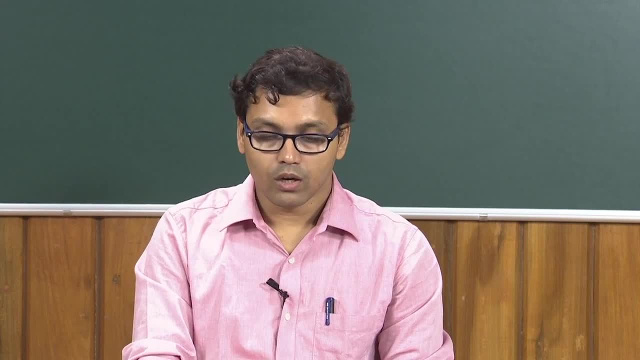 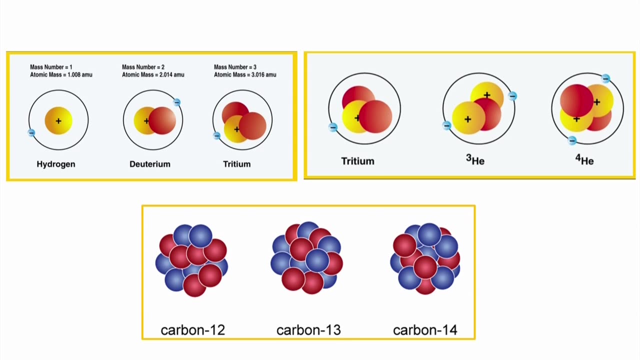 will be only a single electron in the orbits also. These are some further examples of some other isotopes. like carbon can have three common isotopes: C, 12,, 13 and 14. In all the cases you are having six protons. 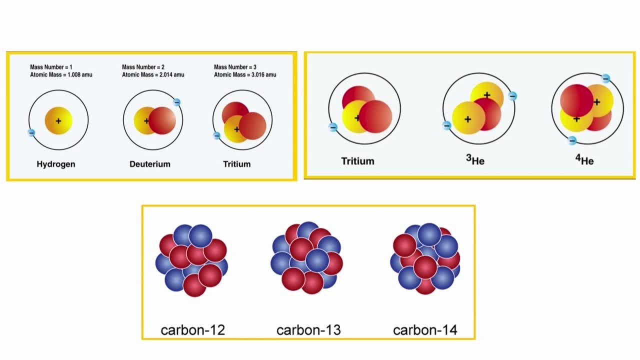 protons in the nucleus, but number of neutrons varies, respectively 6,, 7 and 8.. And as a result of that it is also possible to have the nucleus of 2 different elements which are having different atomic number but the same mass number. For example, just compare tritium, which is the 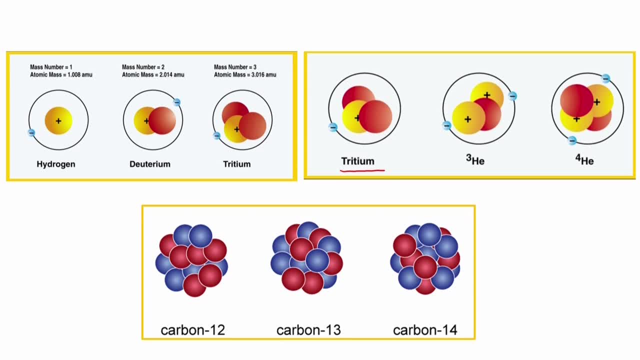 third isotope of hydrogen. having 1 proton and 2 neutron, it is having a mass number of 3.. Now you compare that with 3 helium or 3 He, it is having an atomic number of 2, because there are 2 protons but a single neutron. it is also, therefore having a mass. 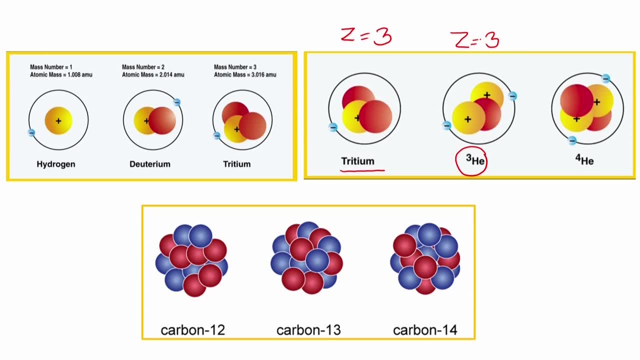 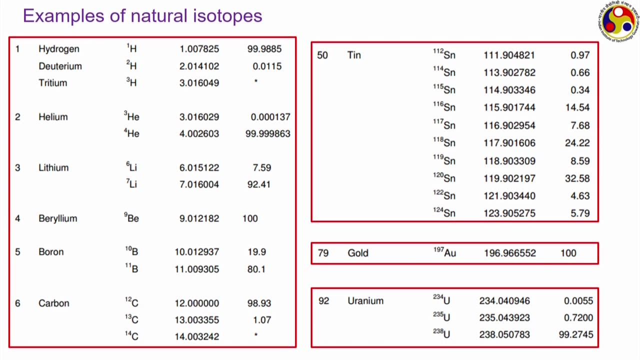 number of 3.. So both tritium and 3 He they are having the same mass number but different atomic numbers. Of course the common isotope of helium is helium 4, which has 2 protons and 2 neutrons. Mostly all natural elements can have several isotopes, like I. 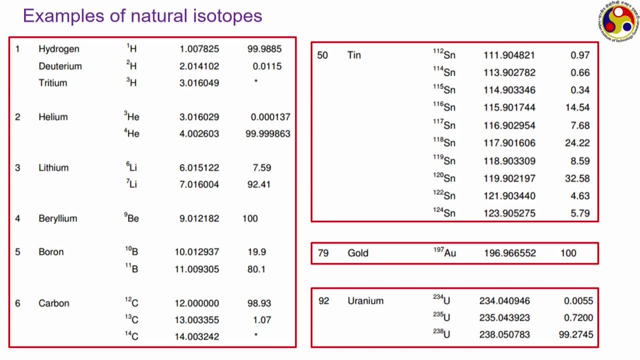 have listed here, some of them: boron can have 2, lithium can have 2.. Some of the substances such as the beryllium or gold, they are having just 1 known isotopes. we can artificially produce several others in the laboratory. 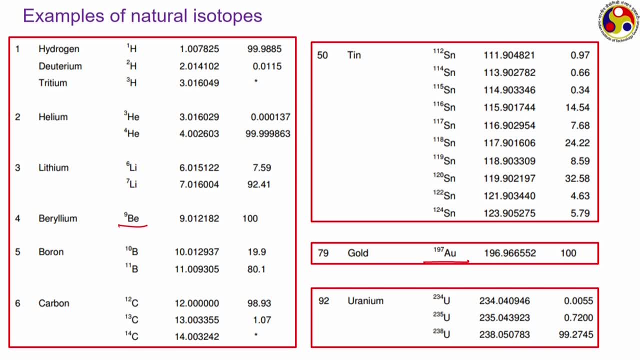 But in nature we generally found only one of them, whereas some of the elements can have several. like you can see here, 14, it has several isotope, isotope starting from mass number of 112 to 124. And all of them are quite prevalent in nature. because you 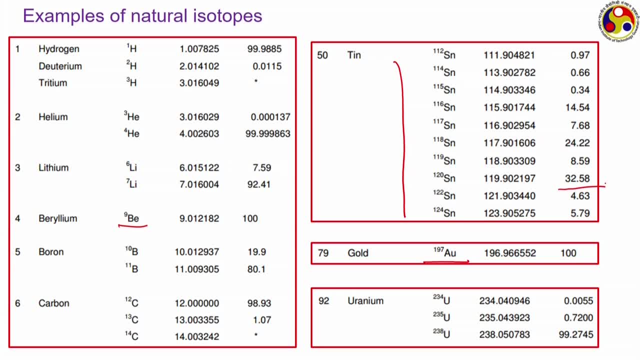 can see where SN 120 appears, about 32 percent, this is also appearing 24 percent and this appears 14 percent. So all of them are quite prevalent in nature And our primary interest here is uraniumureanium commonly has 3 isotopes: U 234, U 235 and U 238, all of them having 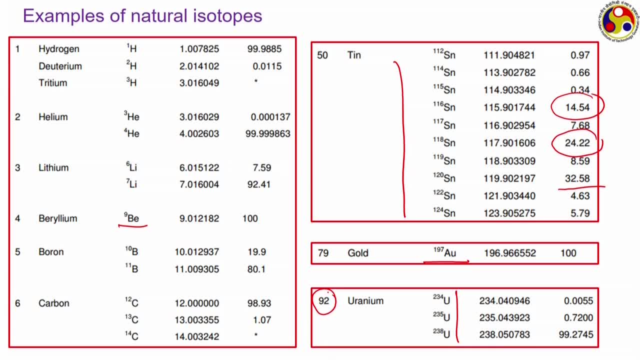 the same atomic number, which is 92,, but the number of neutrons varies. U 238 is the most common one, which comprises 99.3 percent about the of the uranium ore that we extract from the iron, But it also contains very small amount, about 0.7 percent, of U 235 and very little amount of uranium. Okay, So what is the euro in terms of total energy use? S in terms of, though, this coefficient which we can see, it is basically just 0.15.. Detailed, this is equal to 0.15.. So where is the minimum radio? and as if thisまた need to do thisим. 234, little amount of 234. So, ah, different isotopes are. the same element can have different number of neutrons and accordingly their nuclear characteristics can be completely different, like we shall be seeing later on. while the difference between U 235 and U 238 is only.